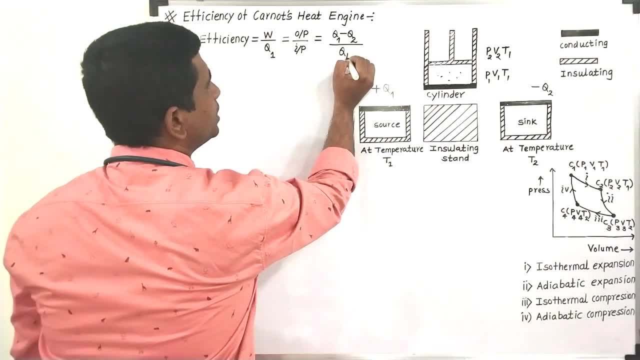 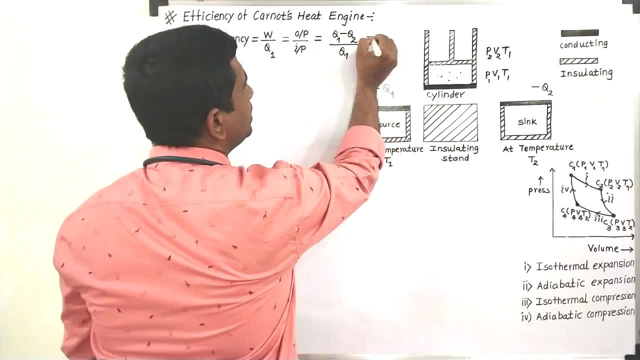 The input amount of heat we have given. It is Q1.. Let us say Q1 is the amount of heat which we are given. If I divide this Q1 by this Q1 and this Q2, I will get Q1. divided by Q1, it will be 1.. 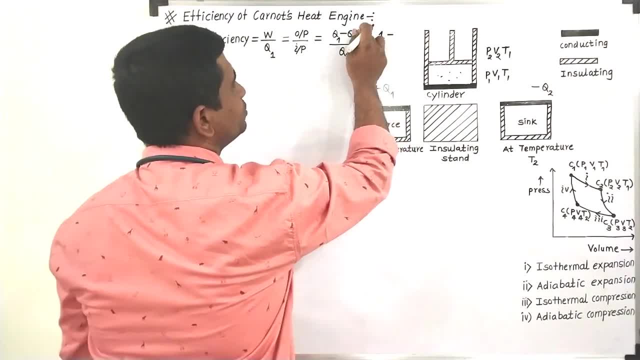 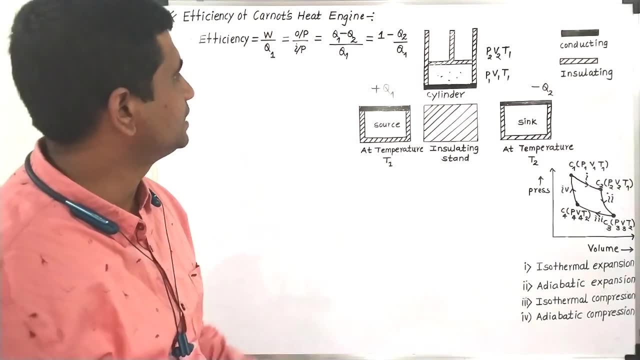 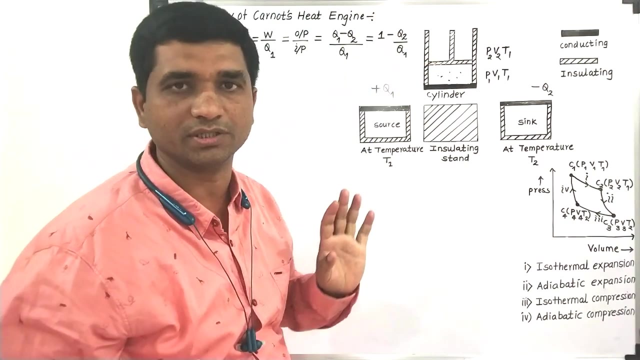 Q1 divided by Q1, it will be 1 minus. this will be Q2 divided by Q1.. This will be Q2 divided by Q1.. From this one what we can say? that the efficiency of a heat engine or efficiency of a cornered engine, it is always less than 100%. 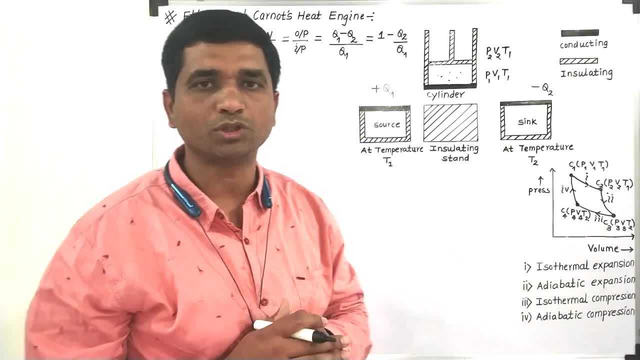 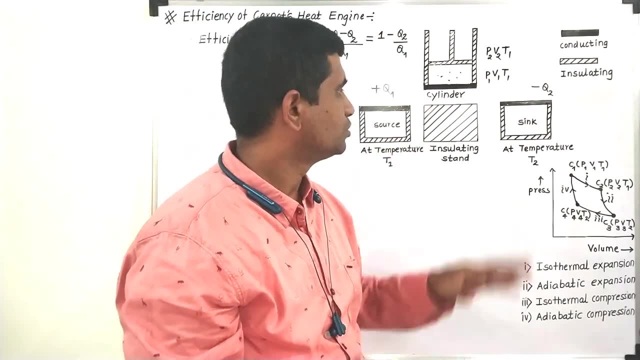 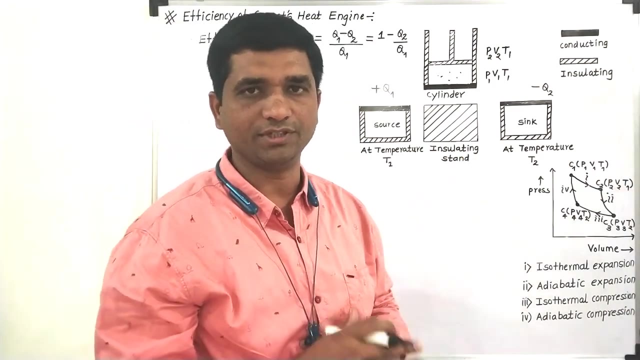 Because some amount of heat will be given to the sink. It is never possible, it is not possible to use 100% amount of heat for work done purpose. okay, So that is the limitations which are having. okay, So you cannot design any machine which can give you the 100% efficiency. okay. 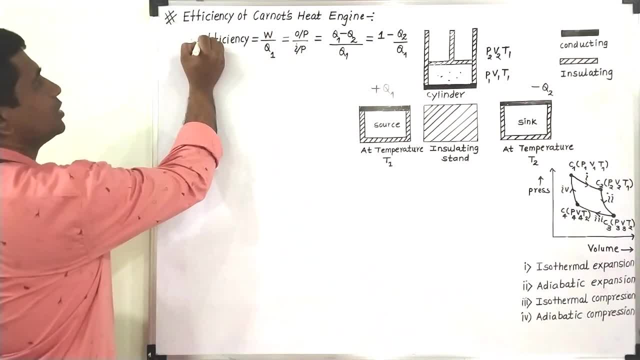 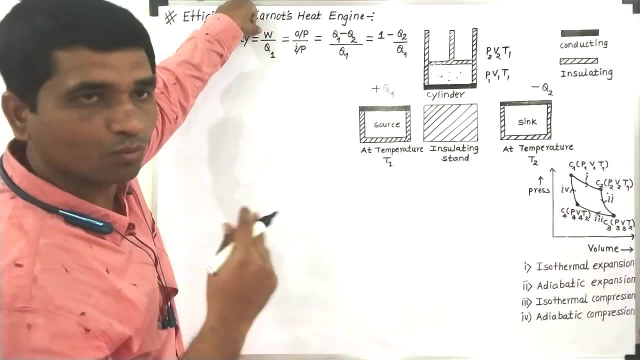 That is the first thing. Now, in order to calculate this efficiency now, in order to calculate this efficiency, what will we be going to use? We have to calculate the work done during the work done. We have to calculate the work done during the work done. 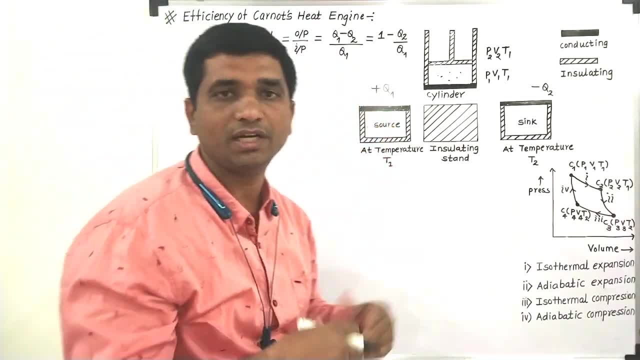 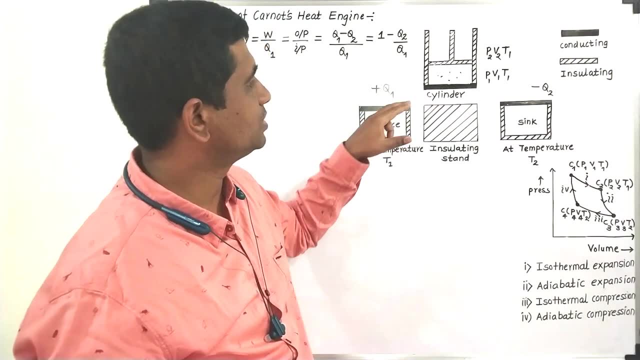 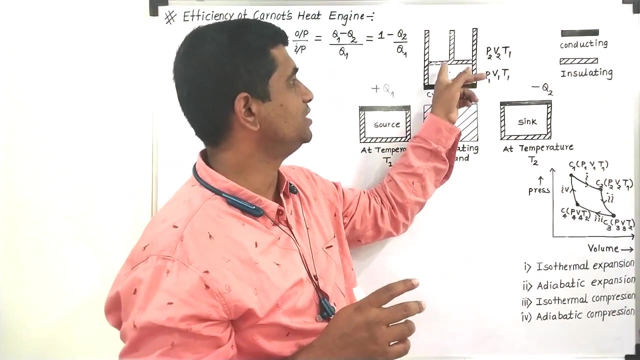 In the all this four processes and divided by the amount of heat given to the system. okay, So the different parts of the cornered engine I have listed over here. The different parts of the cornered engine are: it consists of a cylinder which consists of one mole of an ideal gas enclosed inside this one. 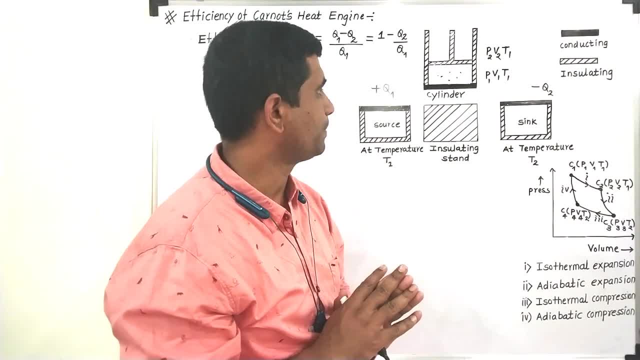 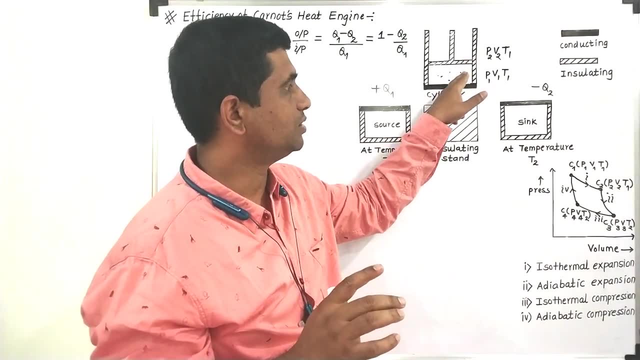 and this cylinder is fitted with a movable, frictionless piston. Okay, So that is the first part, which is a cylinder which contains one more of a perfect gas enclosed inside this cylinder and which is fitted with a piston, which is which can move frictionlessly over this surface. 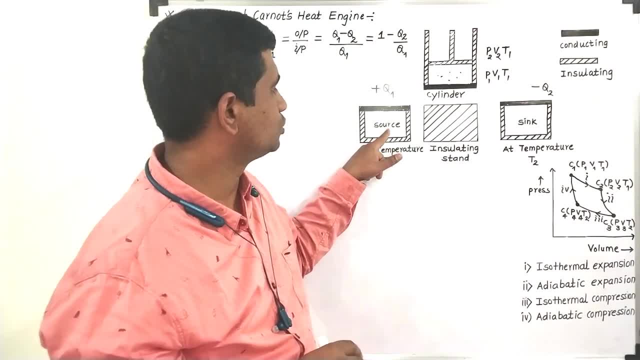 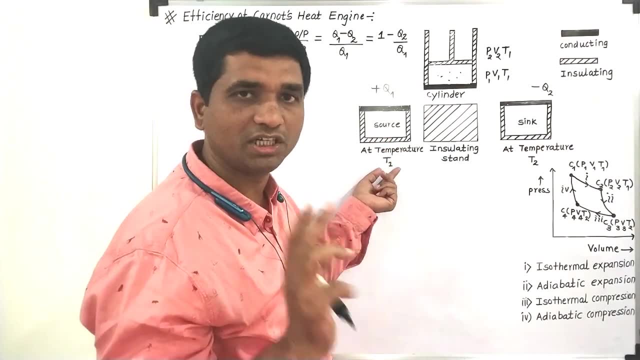 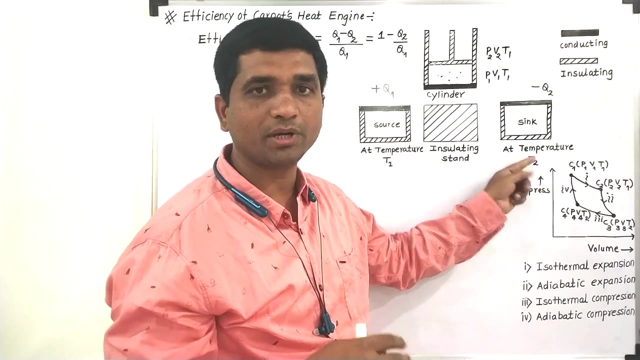 let us say another part of the kernel engine. it is the source, which consists of a heat. it is an infinite source of the heat which is maintained at a temperature t1. okay, this temperature of the source is higher than the temperature of the sink, which is maintained at a normal temperature, t2. so you have to remember that t1 is always greater than. 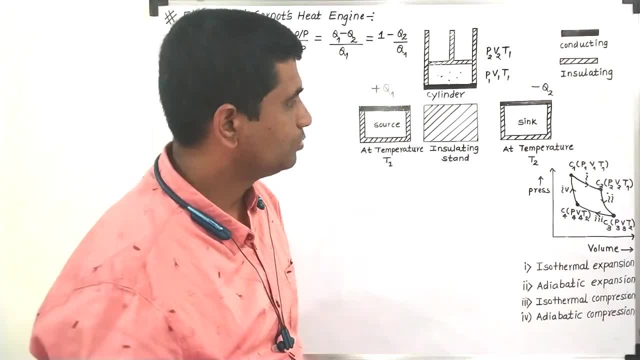 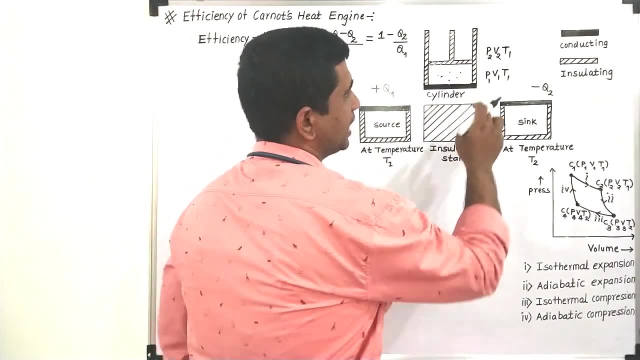 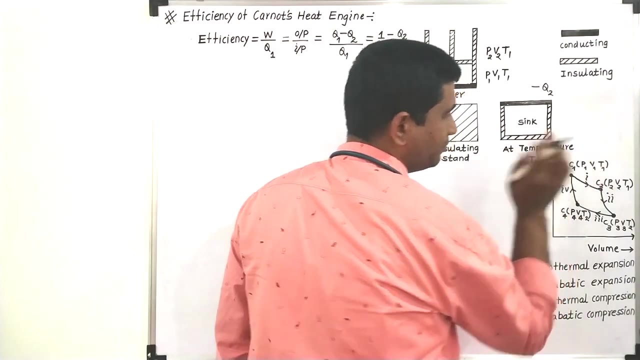 t2 and this is an insulating step. okay, now let us consider that, whatever the gas molecules are enclosed inside this cylinder, so it has a pressure t1, while it has volume v1 and it has temperature t1. okay, so when we are at this point, c1. okay, so we will take this cylinder, we will keep it on this. 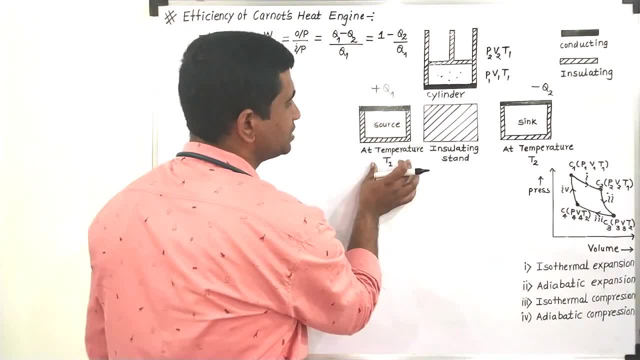 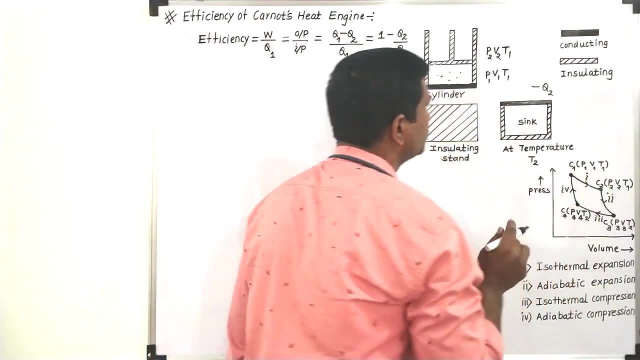 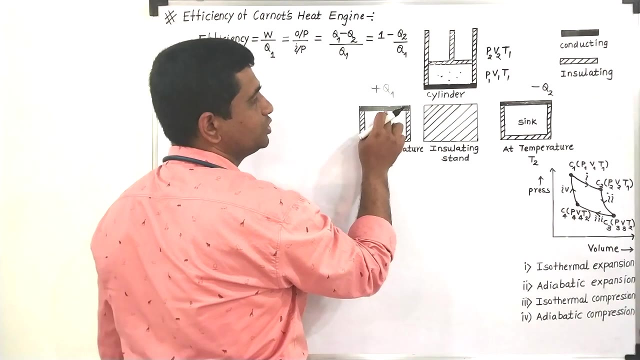 source, okay, source is an infinite source of heat which is maintained at a constant temperature, t1. so when we are starting from this point, when we are starting from this point, as it is a source, lower surface of this cylinder- it is conducting in nature. the upper surface of this source is also conducting in nature. okay, so when? 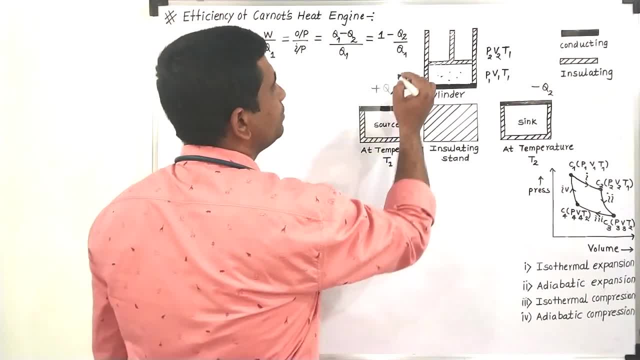 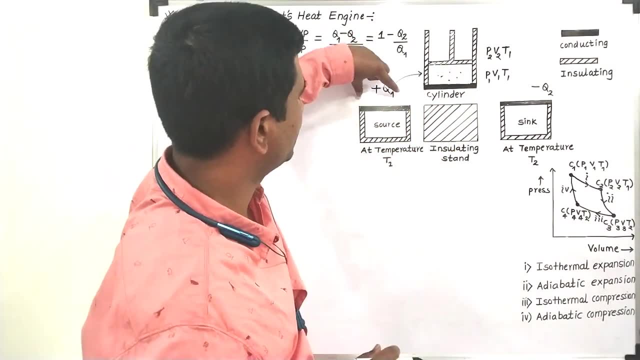 this cylinder is kept on this source, what will happen? it will give a q1 amount of heat to the gas molecule enclosed inside this cylinder. whenever this cylinder is kept on this one, it will give q1 amount of heat to this cylinder now due to that one. what will happen? as the 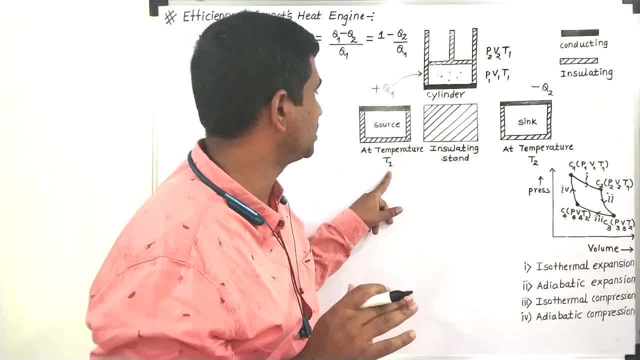 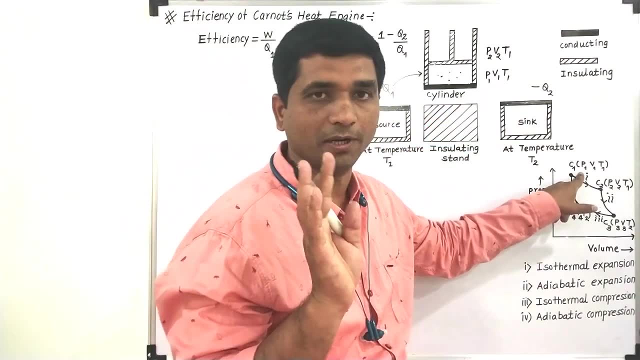 temperature of the source is constant, it has an infinite thermal capacity. so the gas molecules, inside this one, they will attain a temperature t1, so you are at this point, c1. okay, now what we will do. we will adjust the external pressure on this piston in such a way that the gas will expand. 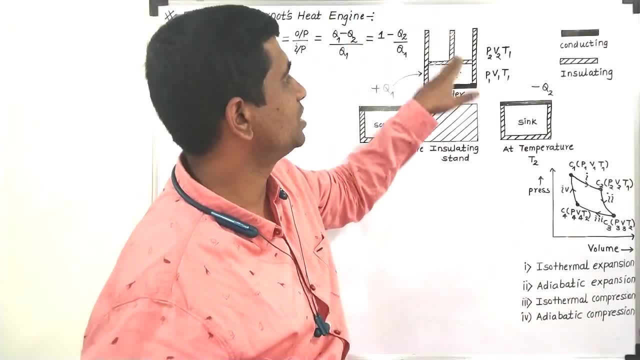 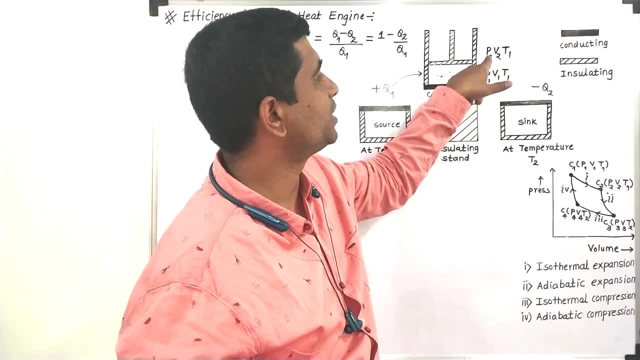 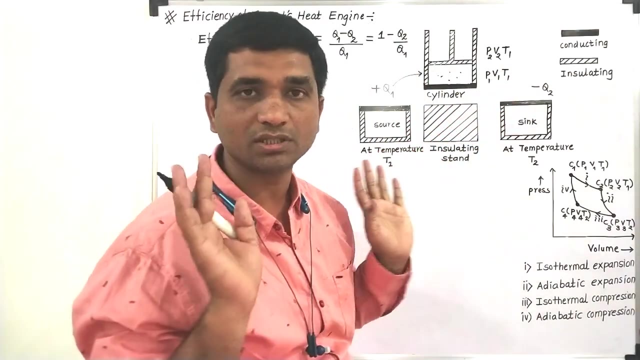 means the piston will move in upward direction. as the piston will move in upward direction. so what will happen? due to that one, the volume will increase from v1 to return. its pressure will, let us say, as it is an isothermal expansion, so temperature of the gas remains constant. so you 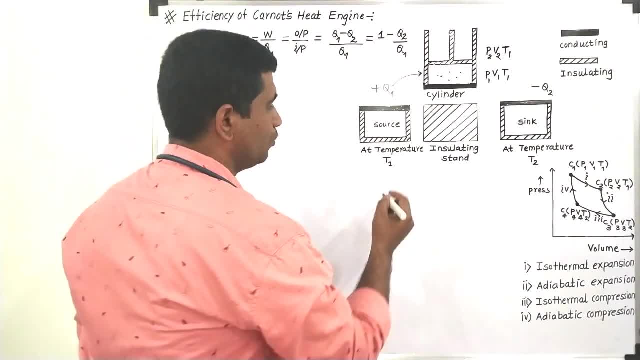 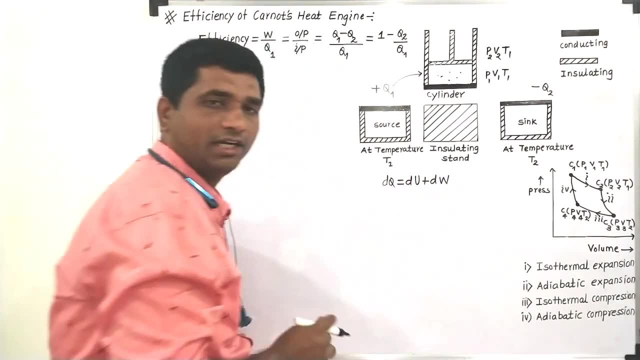 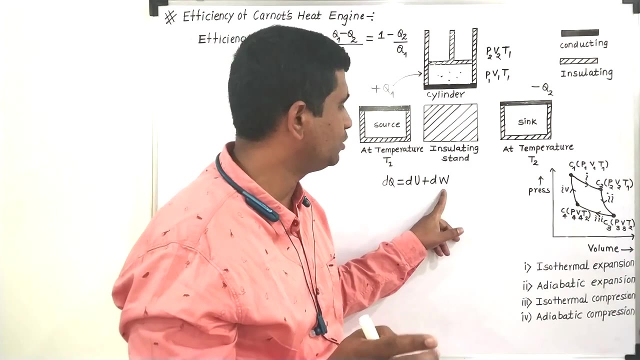 will be getting a some amount of work then during this process. we know from the first law of thermodynamics dq is equal to du plus dw. dq is equal to du plus dw means whatever amount of heat will be provided. it will be used for two purposes: to increase the internal energy and to perform. 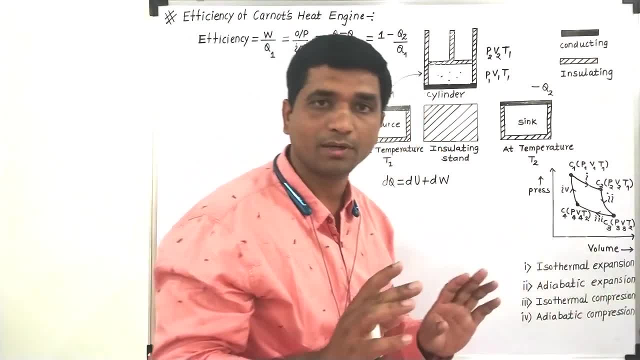 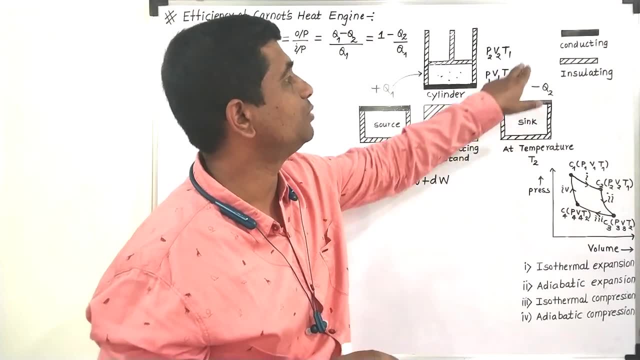 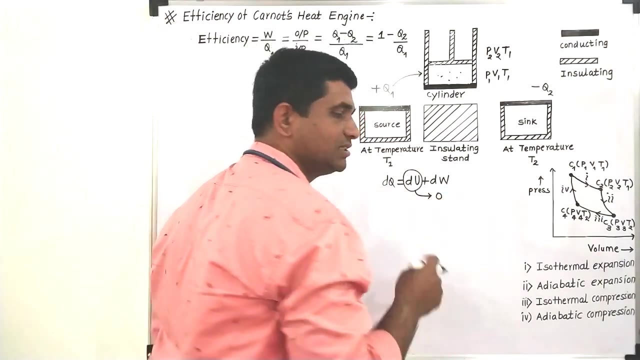 some amount of external work but being an isothermal process, being an isothermal process, the temperature of the system remains constant. temperature t1 to t1. okay, temperature remains constant and we know that the internal energy is a function of temperature. as the temperature remains constant, the internal energy remains constant. so, whatever amount of heat will be provided, it will. 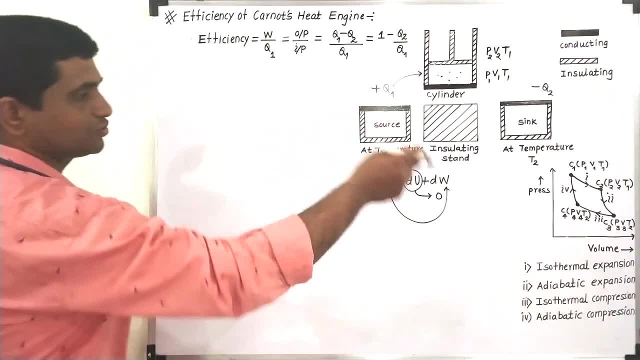 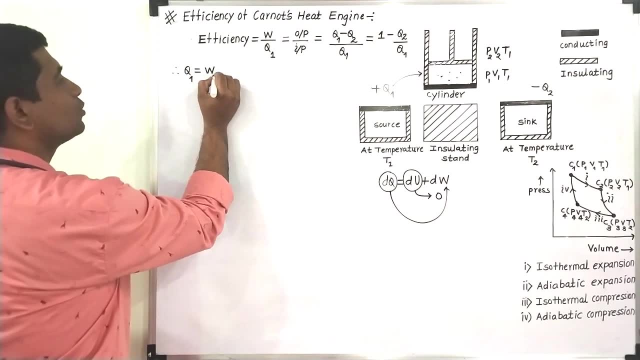 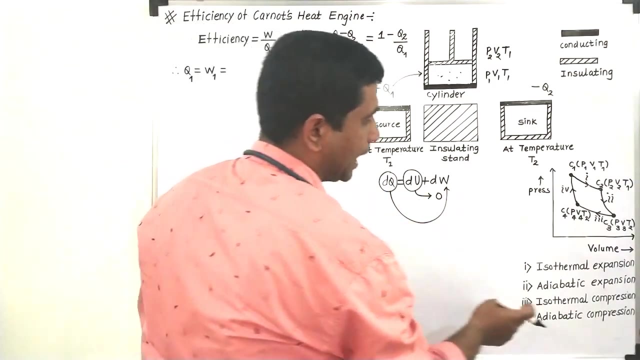 be used only for the work, that means for the first cycle. we can write: suppose q1 amount of heat i have provided and this q1 amount of heat totally will be converted into the internal energy to the work done. from the first law of thermodynamics q1 is equal to w1 and for an 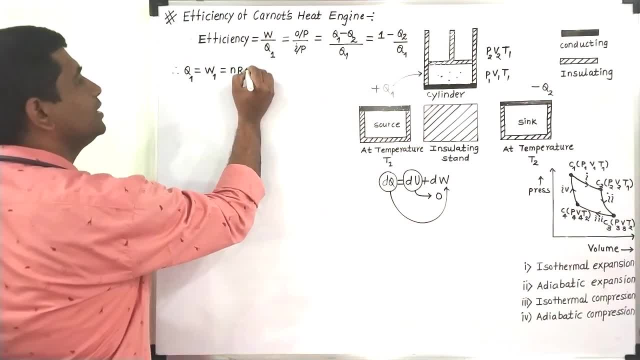 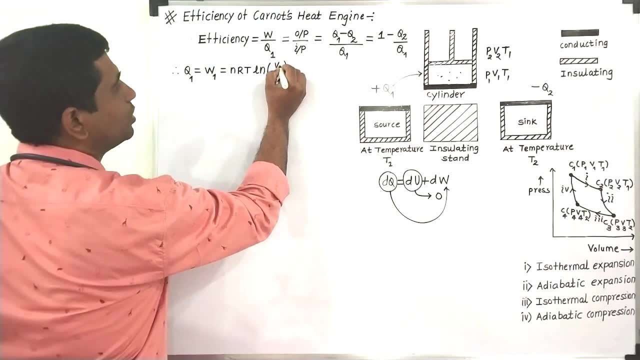 isothermal process. we know the work done. that will be nrt, ln of v2 by v1, ln of v2 by v1. in this case, what is final volume? final volume is v2, initial volume is v1, so it is v2 by v1. temperature of the. 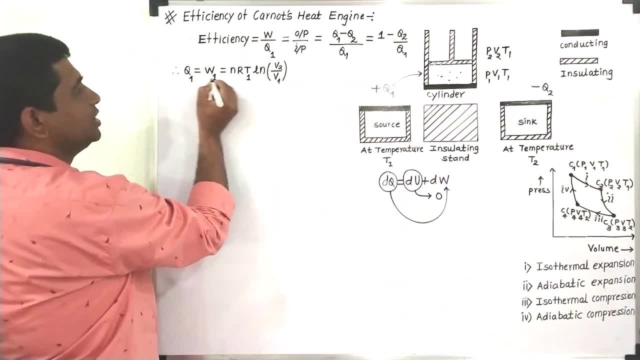 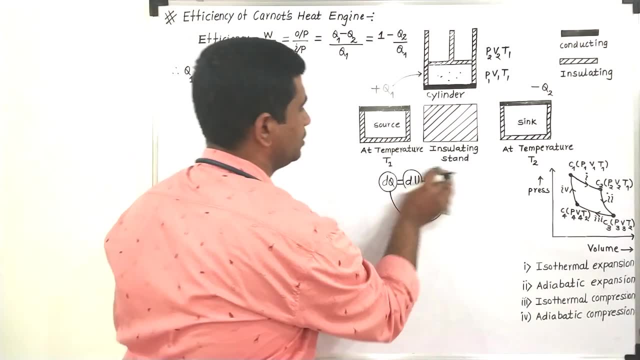 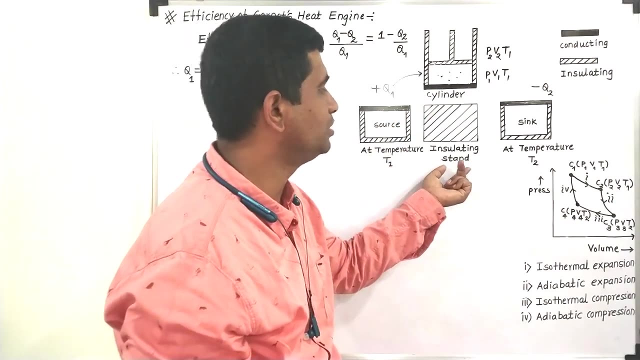 gas is t1, temperature of the gas is t1. so this is the amount of work done we have received for the thermal expansion now in the second step, what it has been done in the second step. now this cylinder is left, left from this source, and it is kept on this insulating stand, the surface of this. 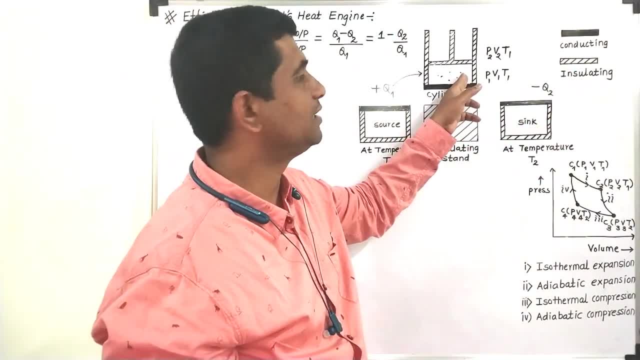 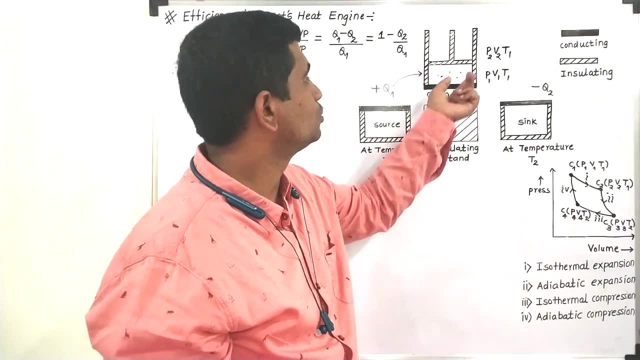 insulating stand. it is insulating in nature, so this cylinder gas molecules which are enclosed in this cylinder, they will not exchange any kind of heat with this insulating stand. okay, so there, in that case, no heat will be given to the system or not taken from the system. so in 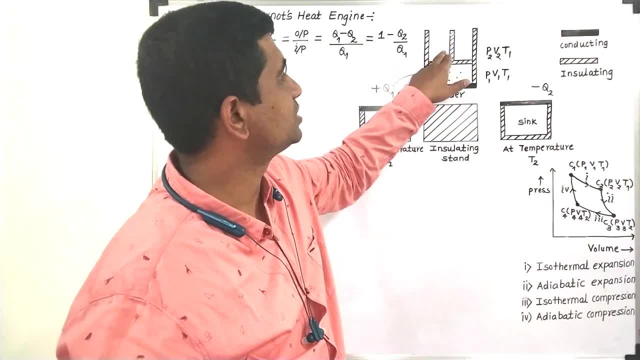 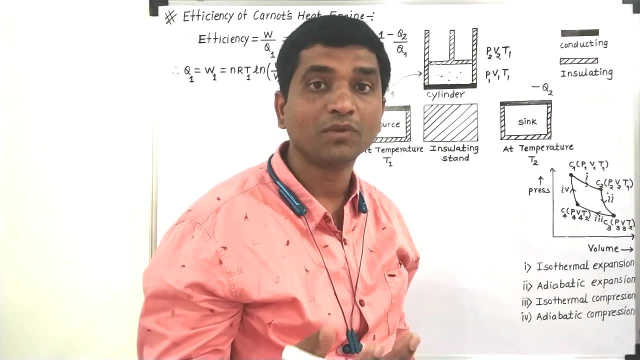 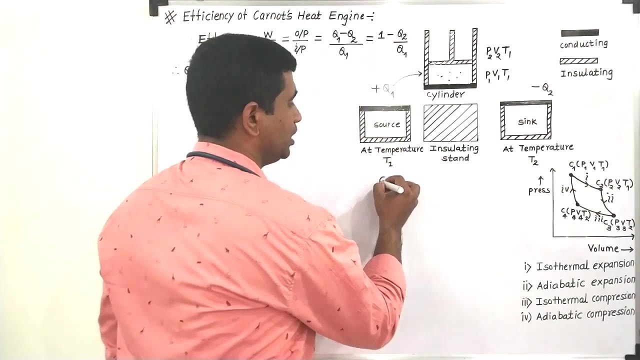 this case the external pressure is adjusted in such a way that the volume of the gas will increase. from first law of thermodynamics we can say that whenever the gas will perform an adiabatic expansion, no heat is provided. so dq in that case it will be zero from first law of thermodynamics. 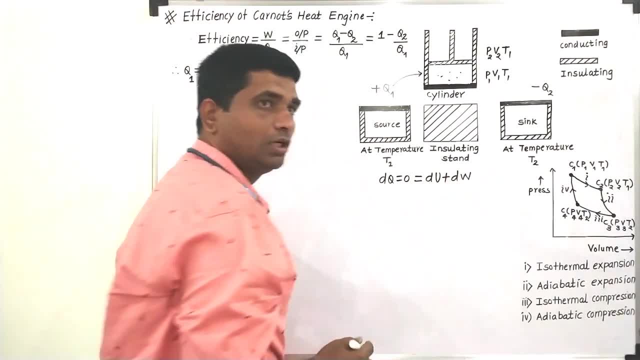 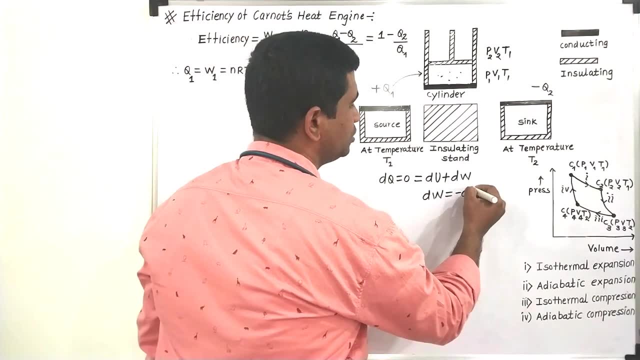 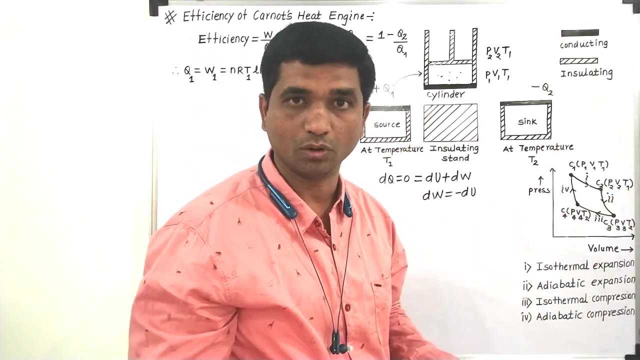 dq is equal to du plus dw. dq is equal to du plus dw. as dq is equal to zero, means whatever amount of voltage it will be there, it is due to the expense of internal energy. means the temperature of the system will fall from t1 to t2. okay, so the temperature will decrease from t1 to t2 and 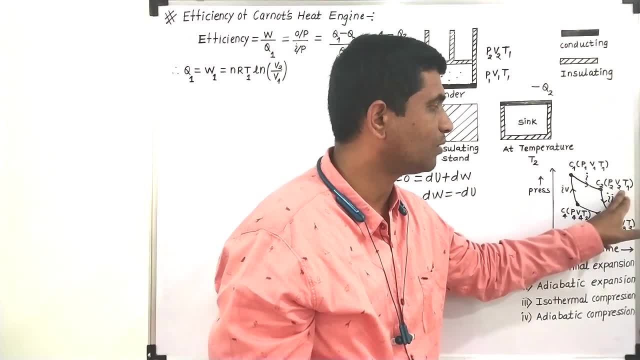 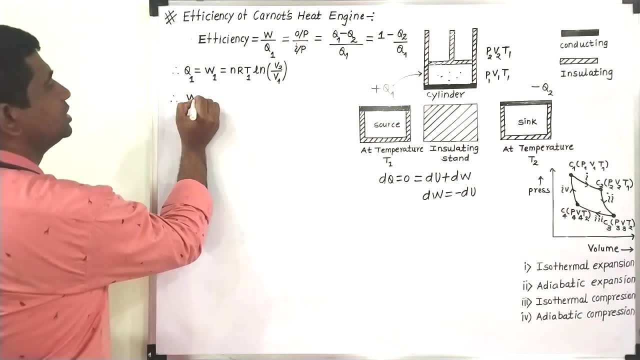 volume will increase from t3, uh volume will increase from v2 to v3. so that is what it is: expansion, and the voltage during such a kind of process, work done during such a kind of process- w2. so voltage will be an adiabatic expansion we had seen in our earlier lecture. 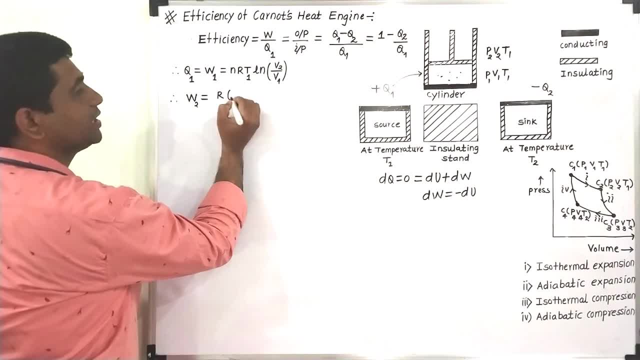 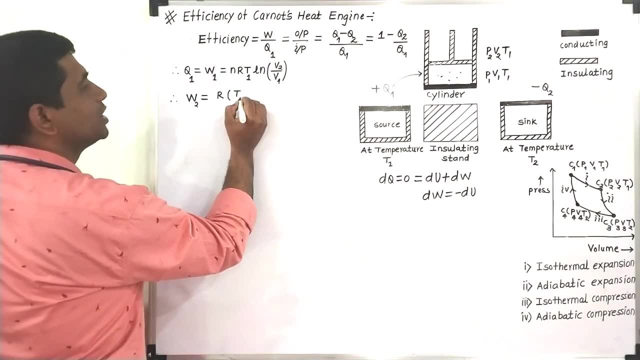 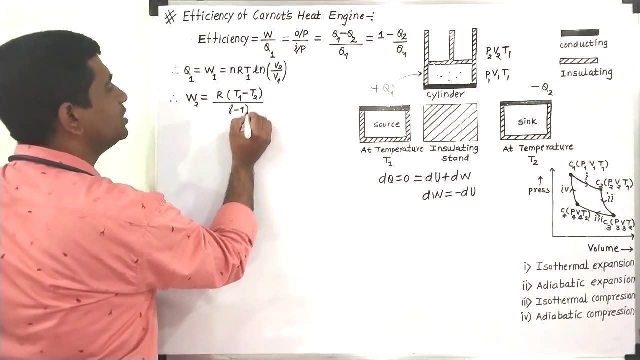 okay, that is nothing but r in bracket, r in bracket initial temperature minus final temperature. so it is: initial is t1, final is t2. so r in bracket t1 minus t2. this will be t1 minus t2 divided by gamma minus one. this is the work done during an adiabatic expansion process. now what we do? now we 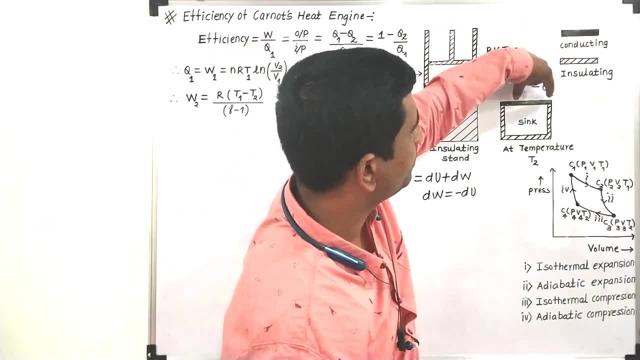 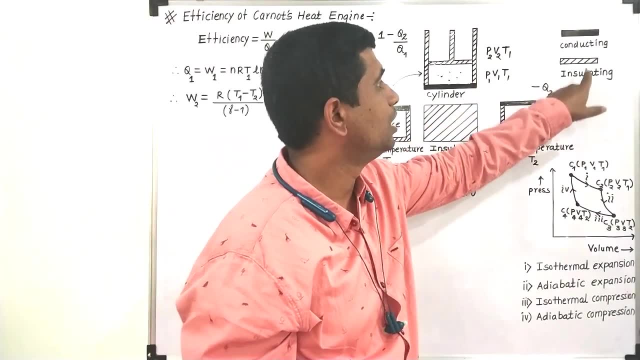 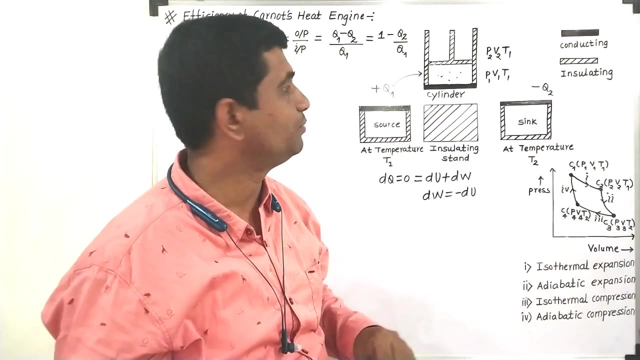 will leave. uh, lift this cylinder from this insulating side. we will keep. keep it on the sink. now the lower surface of the cylinder is conducting. upper surface of the sink is also conducting. okay, so whatever amount of heat, it will be there. whatever amount of heat, it will be there. 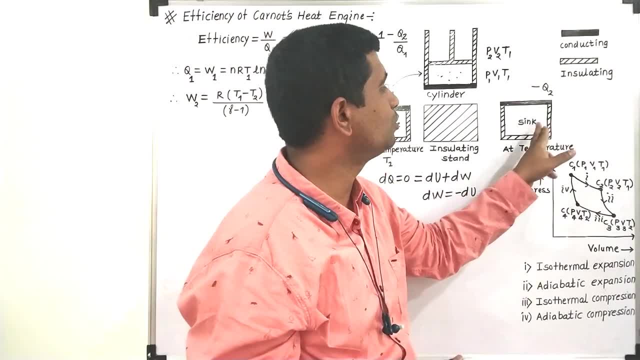 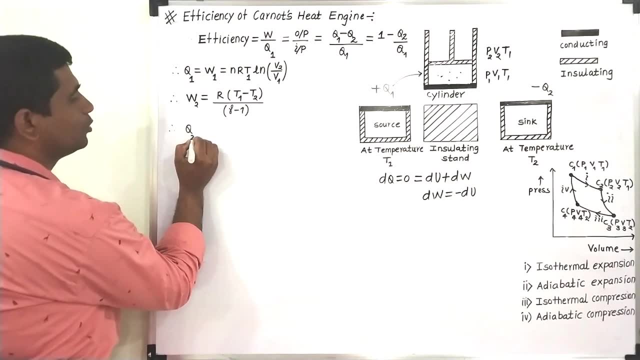 in this gas. it will be unused heat. it will be rejected to this sink because both are conducting. let us say that the amount of heat is rejected to the system. okay, cube, one of heat is rejected to the system and in this case the sink is maintained at a temperature t2. 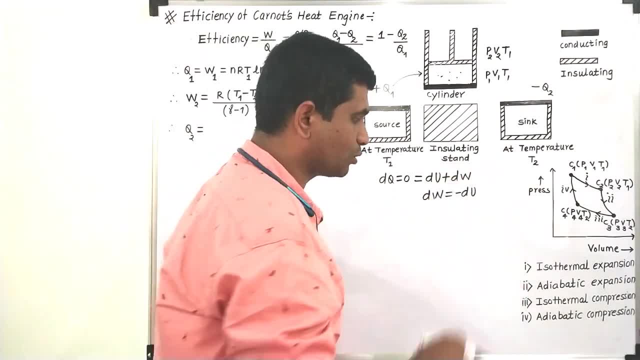 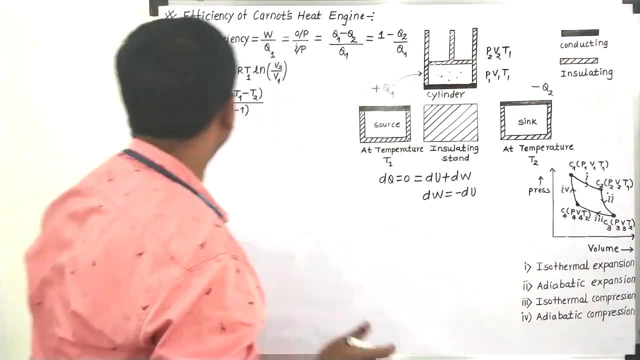 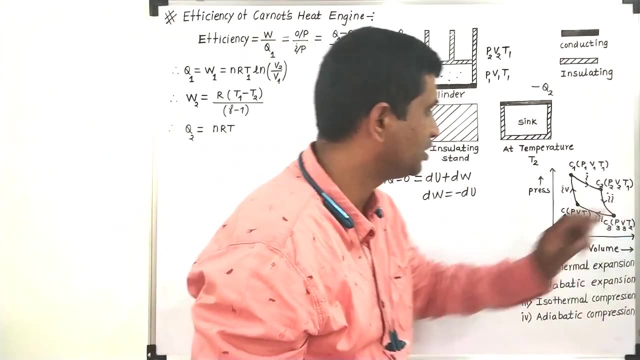 temperature, T2, and so in this process temperature remains constant. so it is an isothermal compression. we will be adjusting the pressure in such a way that the gas will compress. okay, so whole time during an isothermal process it will be nRT, in this case temperature of the gas. 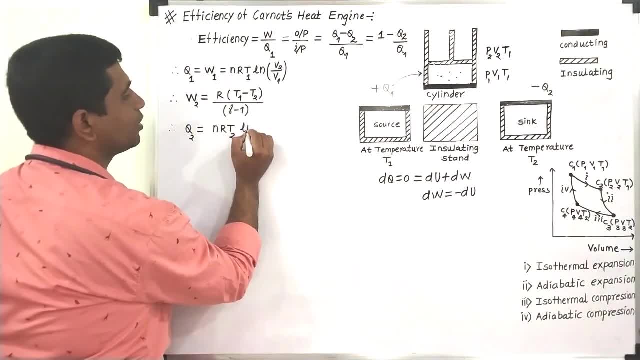 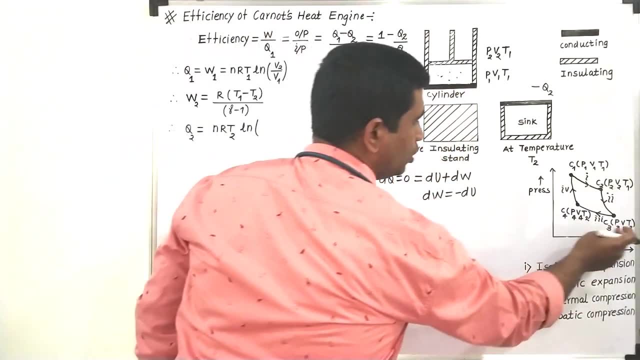 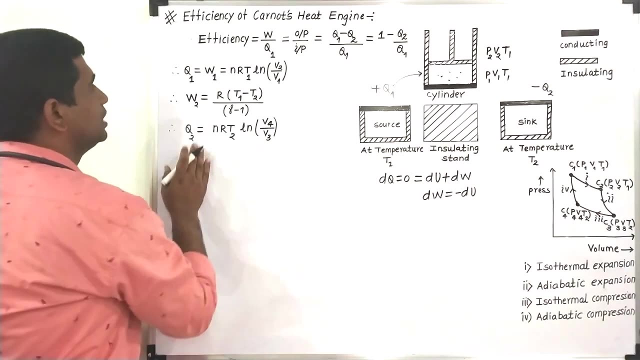 it will be T2, so it is nRT2, nR and where volume is decreasing, our volume is decreasing from V3 to V4, so it is final volume divided by initial volume, so it is V4 divided by V3. so this will be the work done during the third case, so we can write this as a Q2 is equal. 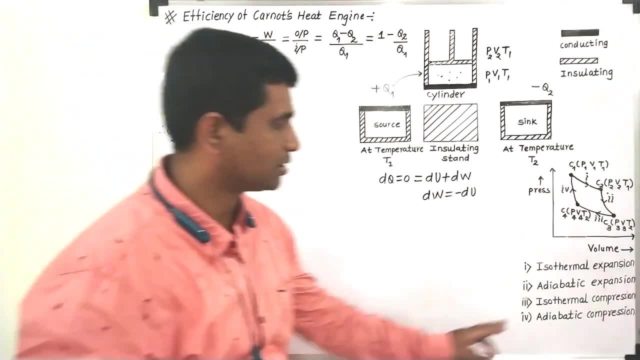 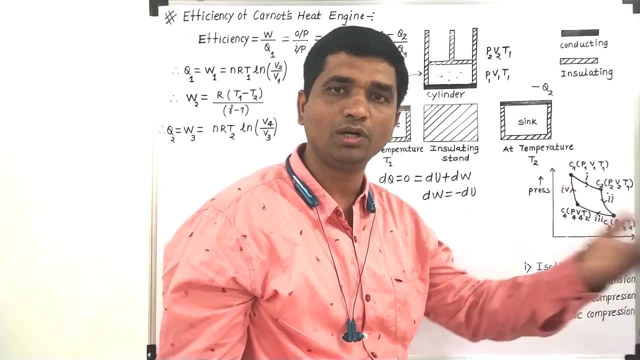 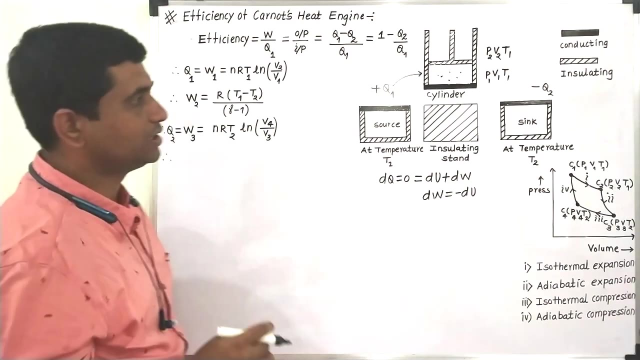 to W3. okay, because, being an isothermal process, internal energy change will be 0, so whatever amount of heat will be given to the system, that will be only converted into the work. okay, so that is there. And now Okay In the second case, in the final stage, this cylinder is lift from this sink and it is 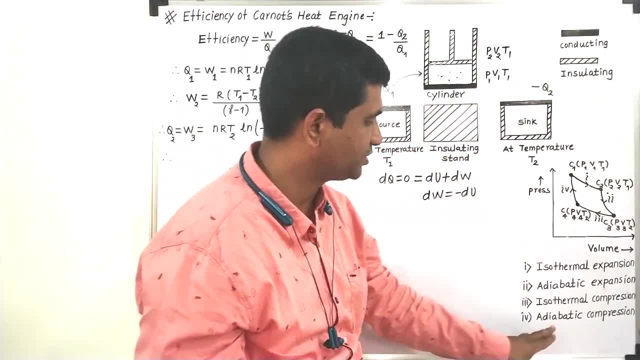 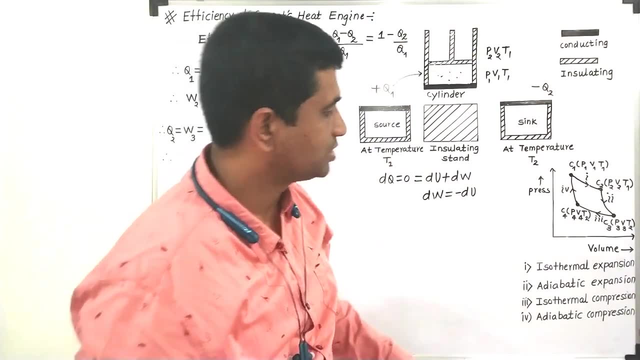 again kept on this insulating stand so that there will be no heat exchange. so it is an adiabatic process and again the pressure on pressure is adjusted such a way that the gas will compress. so let us say that your pressure goes from V4 to V1, volume goes from V4 to 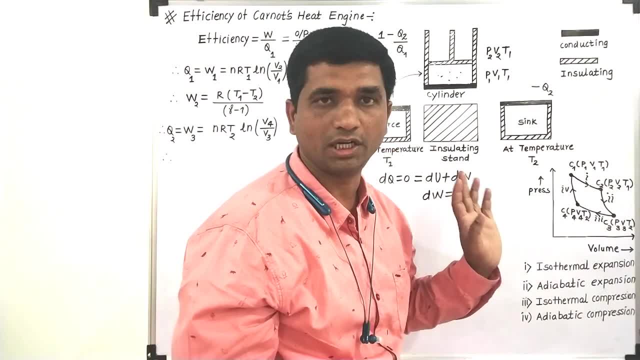 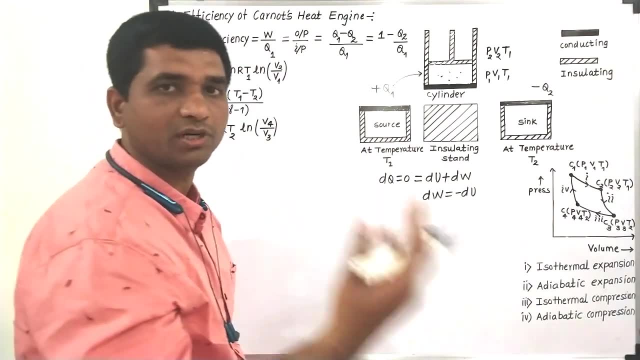 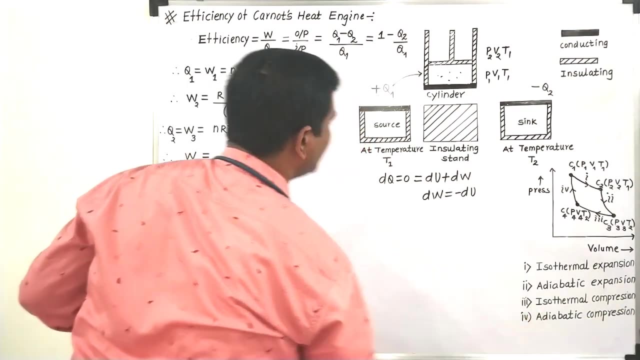 V1 and temperature decreases from T2 to T1. okay, so sorry. temperature increases from T2 to T1 because it is a compression. during the compression, temperature of the gas decreases. so work done, which we will be getting. W4 is equal to being an adiabatic process, so work. 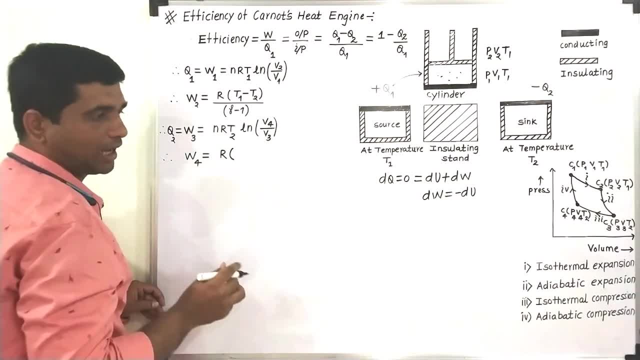 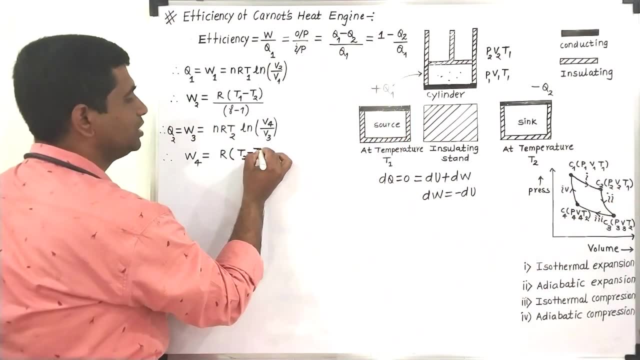 done during adiabatic process. it is R in bracket, R in bracket. this will be initial temperature minus final temperature, so that will be T2 minus T1, T2 minus T1 divided by gamma minus 1, so this will be the work done. 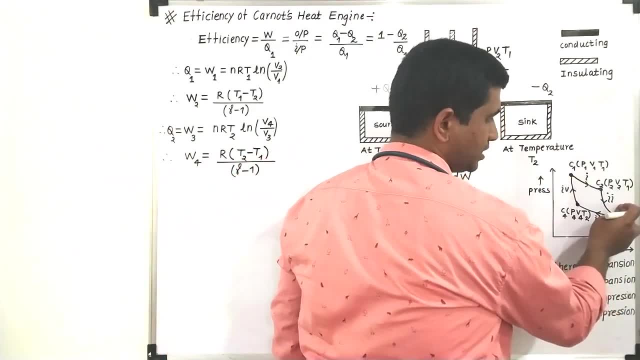 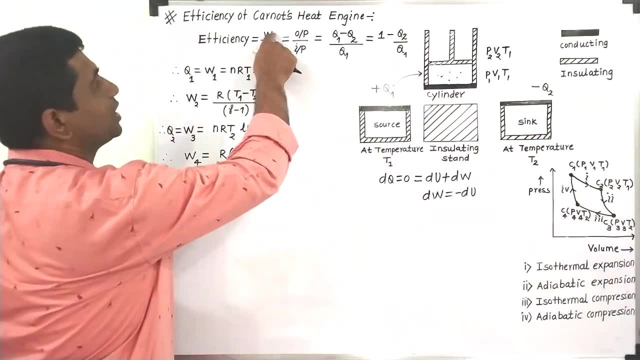 Okay, Okay, Okay Okay. This will be the total work done: W1 in the first case, W2 in the second case, W3 in this case and W4 in this case. now, what I want to do is that I want to calculate the total. 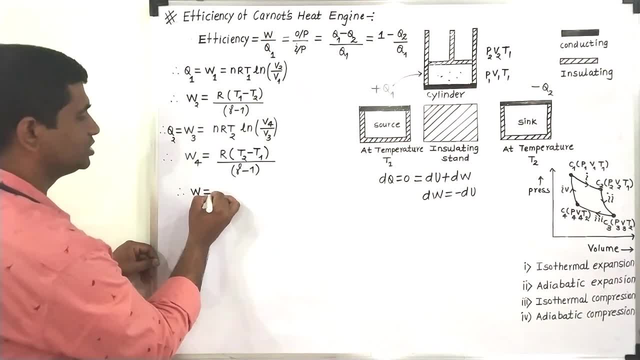 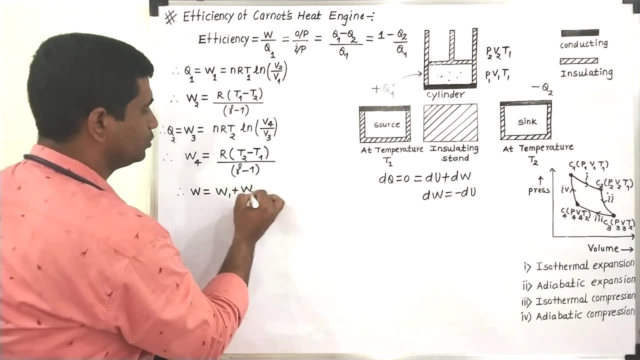 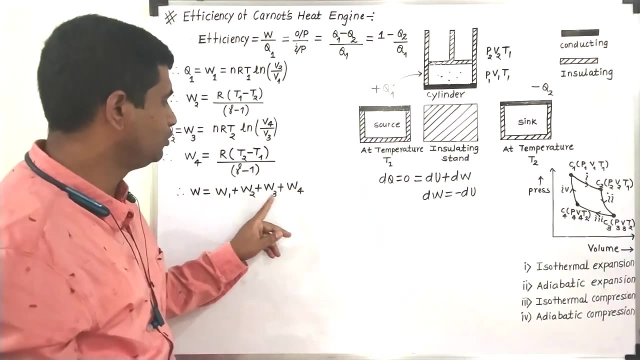 work done. so how we will calculate the total work done? W is equal to. it will be the sum of all these work done, so it will be W1 plus W2 plus W3 plus W4, so it will be the total work done: W1, W2, W3, W4. 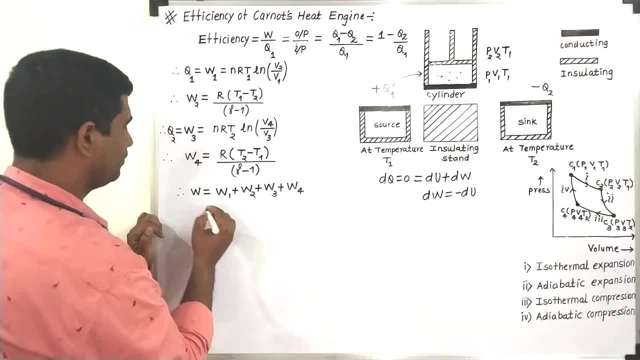 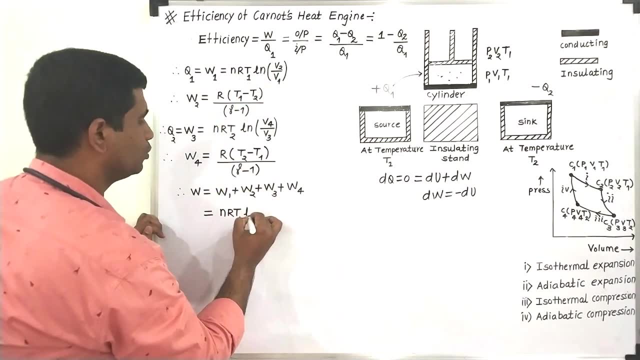 W4. It will be total work done. so now what we will do, we will just try to substitute those values. it will be NRT1, ln of V2 by V1, ln of V2 by V1, plus work done. W2: it will be R in bracket. 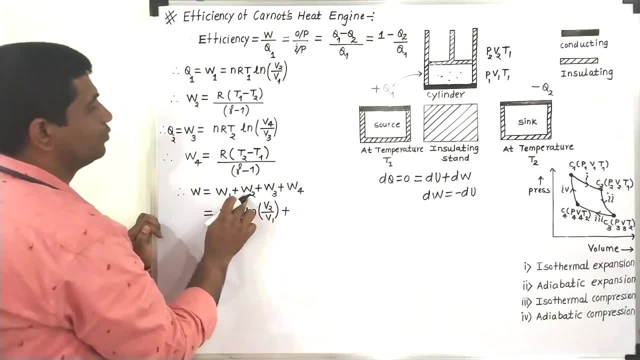 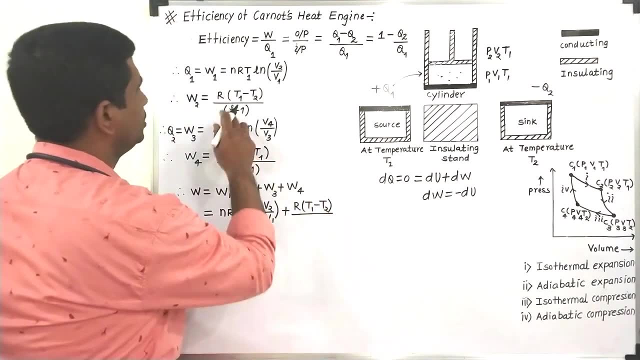 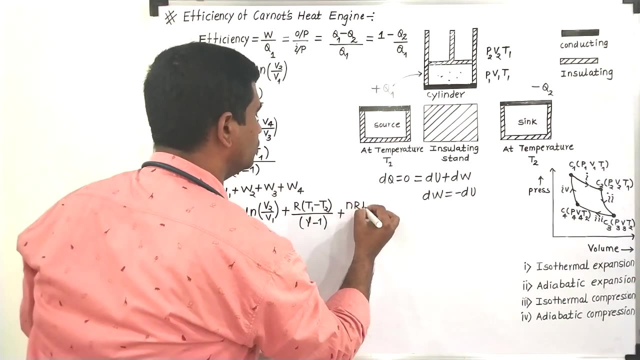 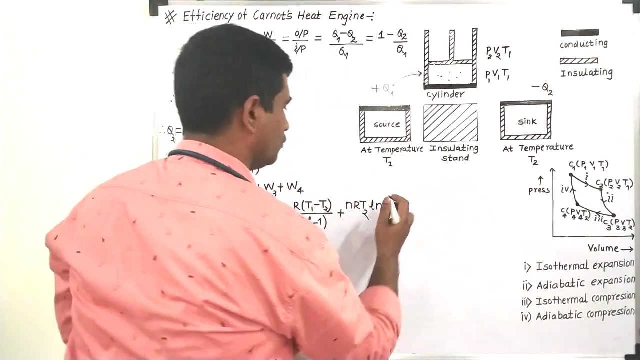 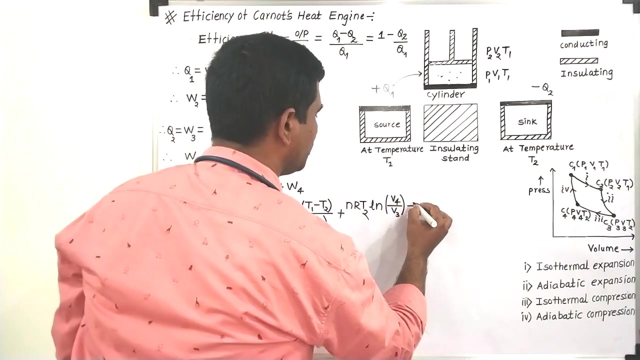 T1 minus T2, T1 minus T2 divided by sigma minus 1 plus W3.. It will be NRT2 if you use more simple measures. Okay, p2: ln of v4 by ln of v4 by v3, so it will be v4 divided by v3, bracket complete plus. 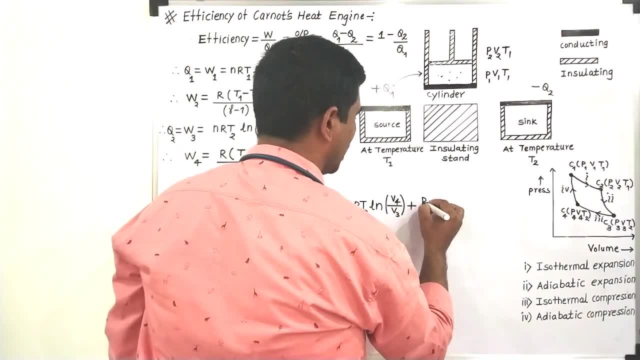 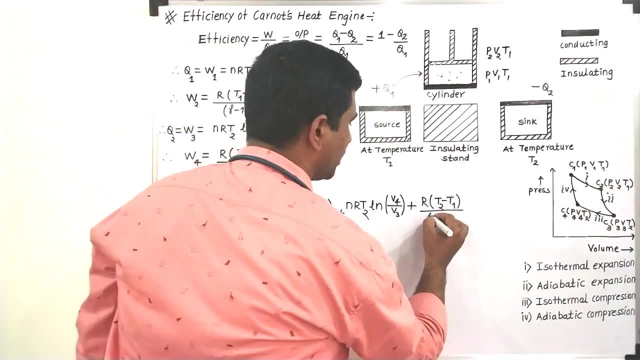 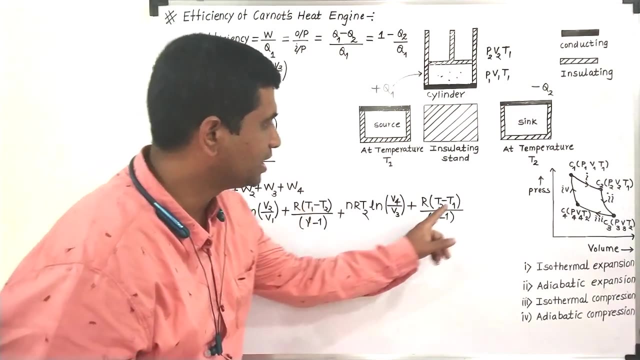 last w4 is r in bracket, r in bracket t2 minus t1, t2 minus t1 divided by gamma minus 1, divided by gamma minus 1, now see here: in this case t1 is positive, here in this: 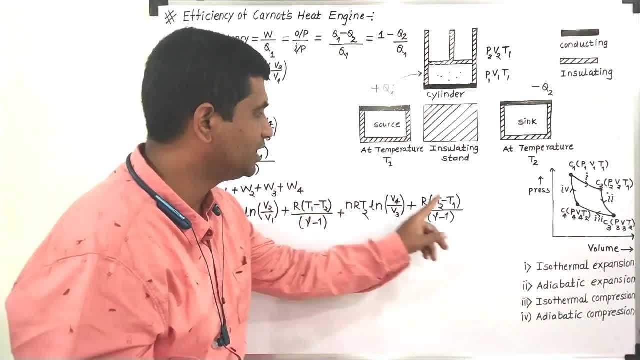 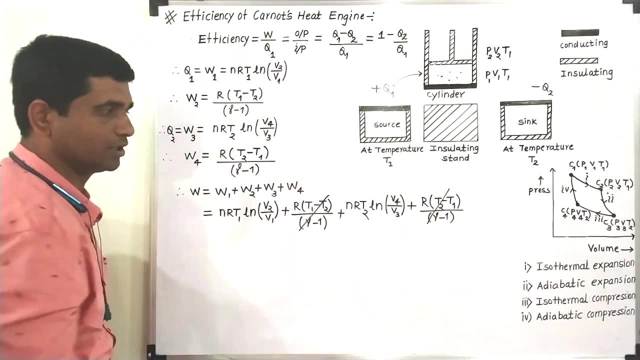 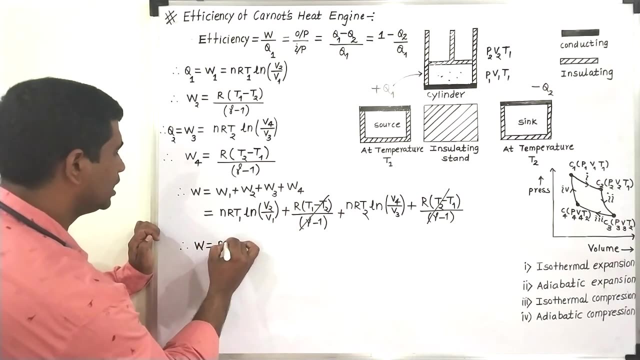 case: t1 is negative. here t2 is negative. here t2 is positive. denominator is same. this r is same means this second term will cancel with this fourth term. so these two terms will cancel each other and therefore w you can write: w is equal to ln of v2 by: 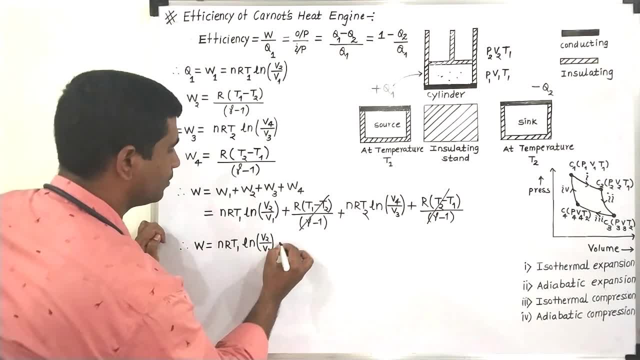 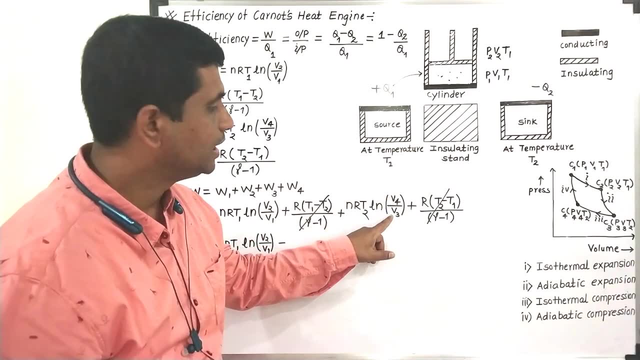 v1,, v2 by v1, plus now here. in this case we have to assume we just take a reciprocal of this one, v4 by v3,. instead of that I will try to write down v3 by v4, so if I do, 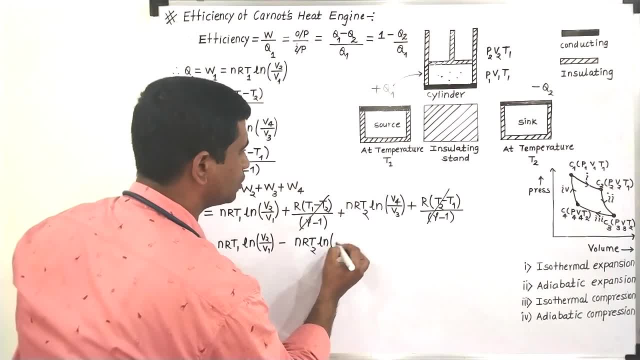 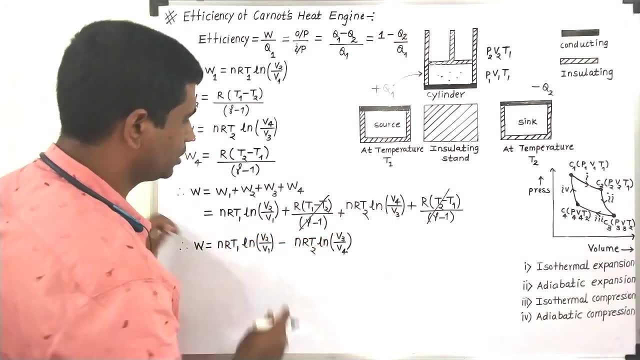 that nr t2 ln of instead of v4 by v3, if I write v3 by v4,, instead of that, if I write v3 by v4, and then I have to take a. I have to make this negative sign as a this positive. 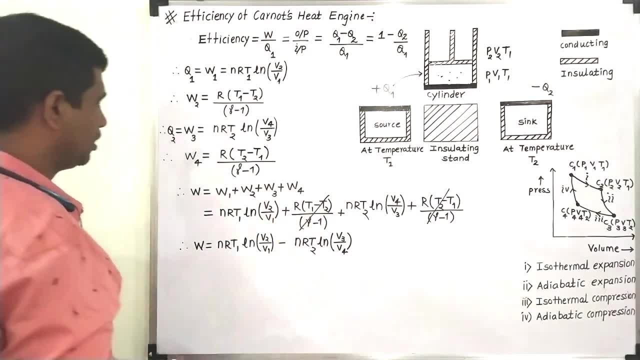 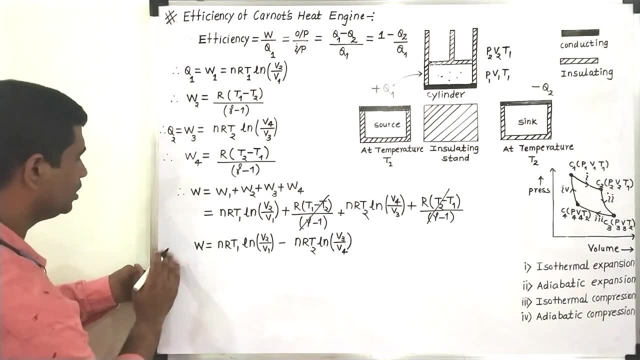 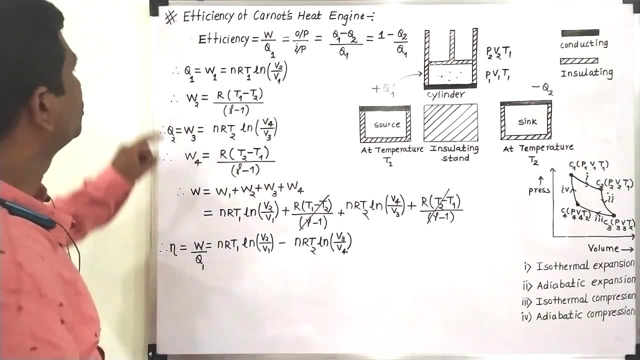 sign as a negative sign. okay, so this is the work done. now how do we define? how do we define the efficiency? it is w by q1, so within this equation only I will just try to write down: eta is equal to w by q1, w by q1, so what is value of q1, it is this. 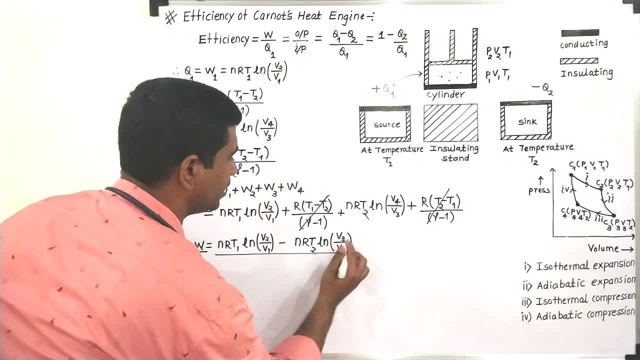 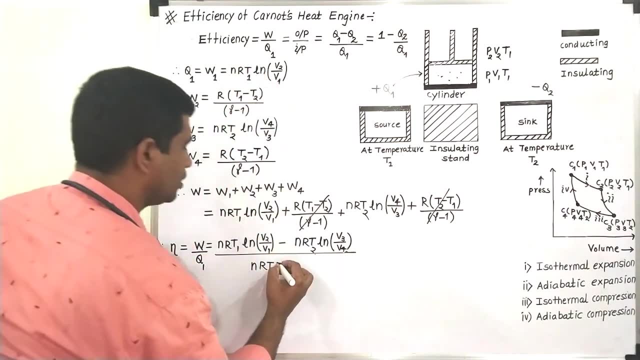 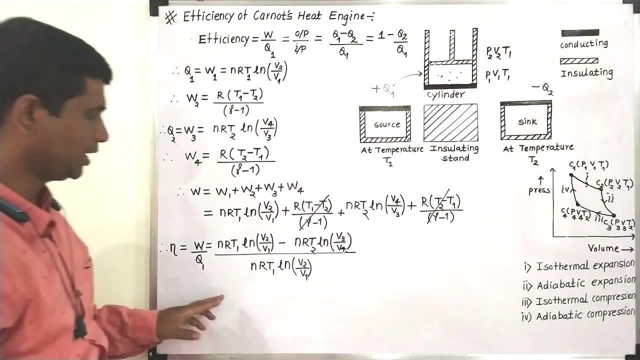 one. so I will divide this expression by. I will try to divide this expression by q1,, which is nr t1.. ln of ln of v2 by v1,. ln of v2 by v1,. okay, so this is the work now from the numerator. 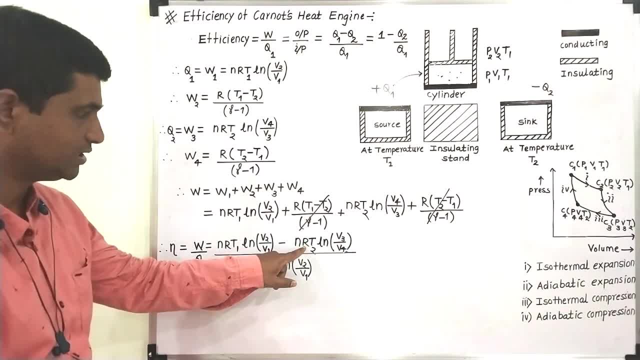 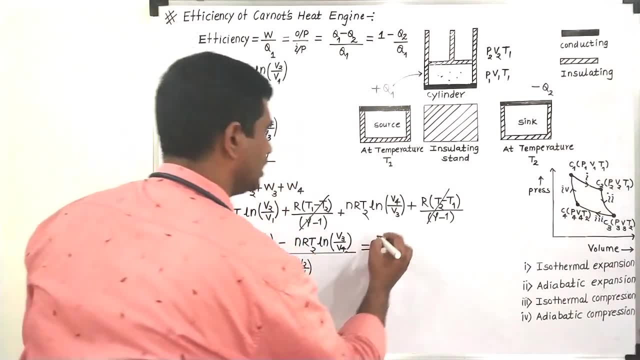 what we can do. we will take this nr common. we will take this nr common. we will take this nr common. they will cancel each other. they will cancel each other. so finally, we will be getting our nr will take common. this nr. we will take common. this will cancel with. 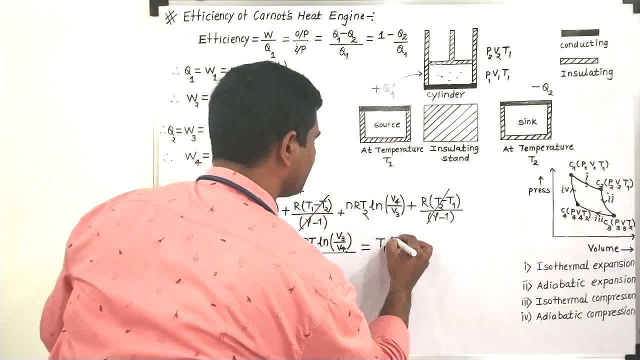 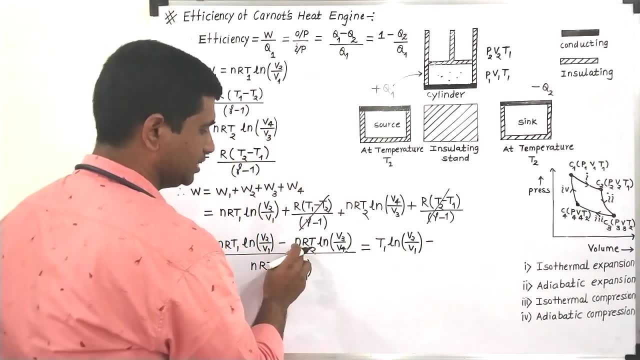 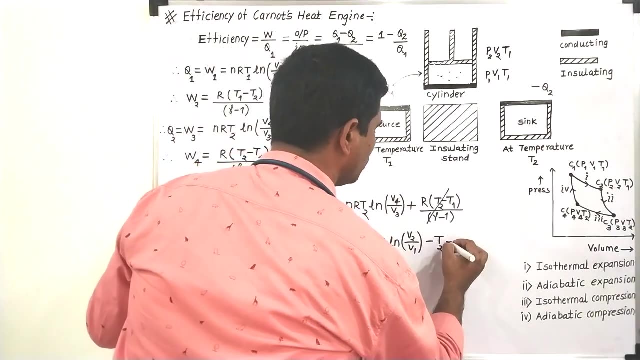 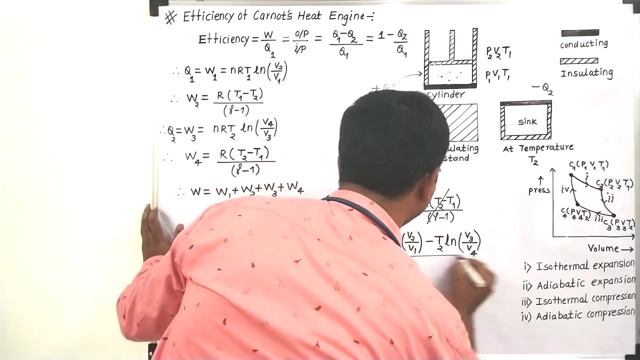 this one. so what I will get over here. it will be t1.. ln of v2 by v2 by v1, that is the first bracket minus nr. we have cancelled, so it is t2, t2, in bracket ln of t2. ln of this will be v3 by v4, this will be v3 by v4, divided. 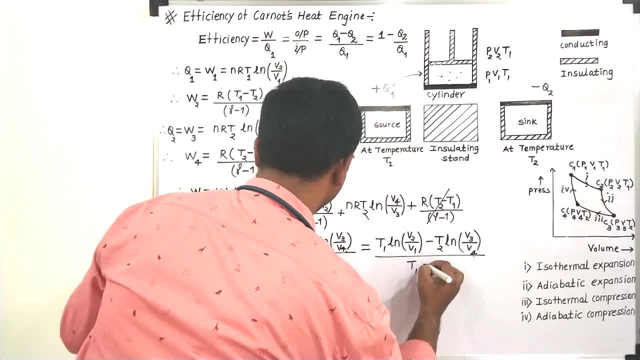 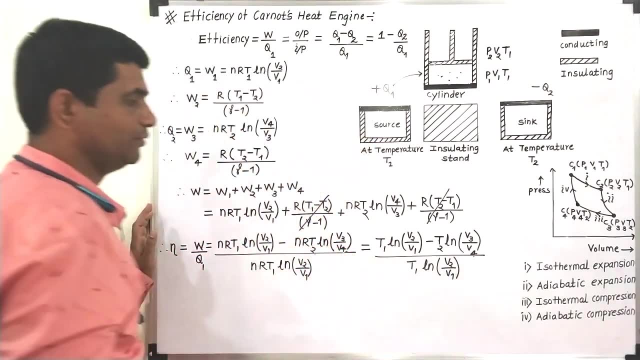 by, and the denominator. we will be getting t1, ln of t1, ln of v2 by v1, this will be v2 by v1, let us call this as an sum equation. let us call this as an equation number 1,. 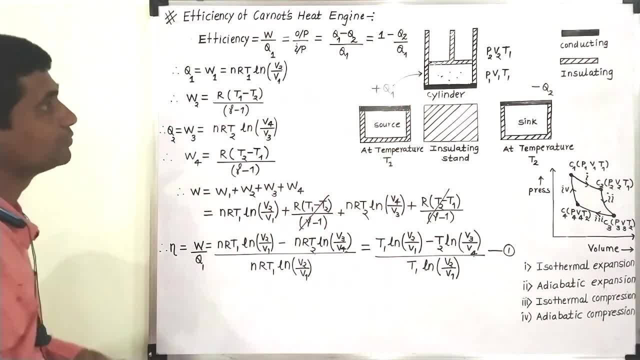 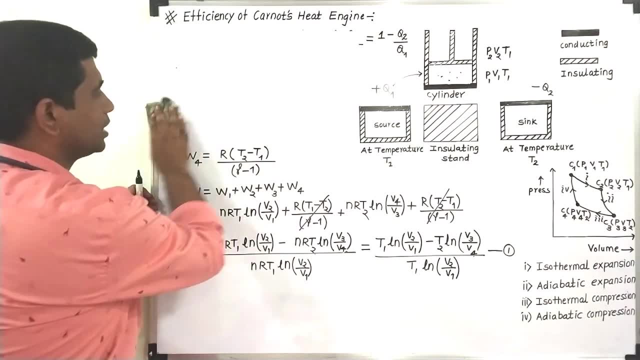 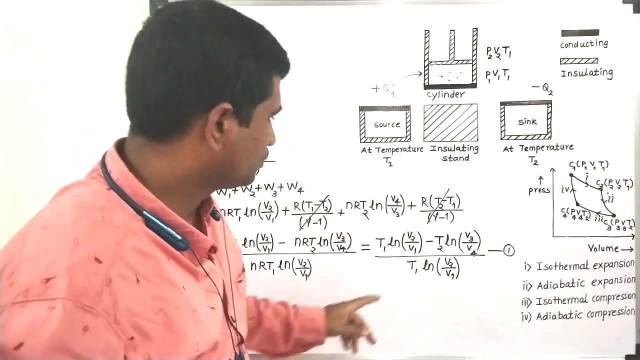 okay, let us call this as an equation number 1, now for what I will do instead of this. I will try to write down at this. okay, over here, I will try to write down now. okay, now let us see. in this case, we have to now simplify v2 by v1 and v3 by v4, okay, v2 and. 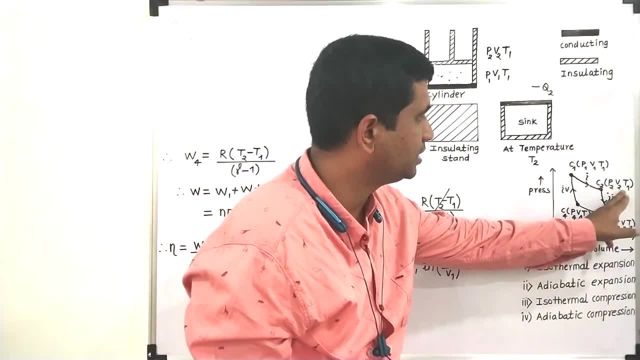 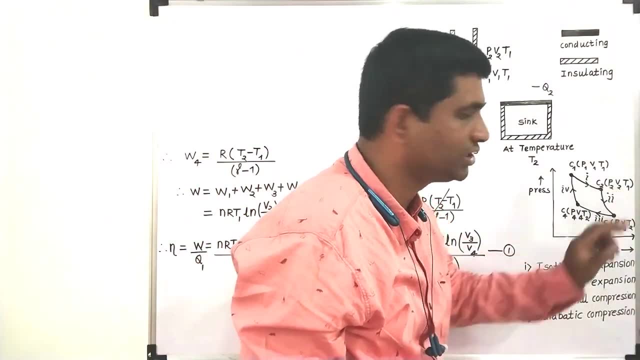 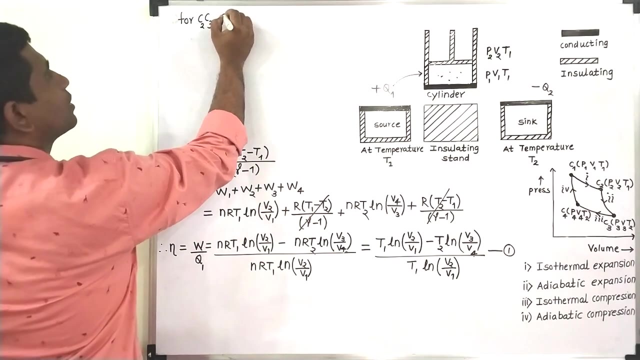 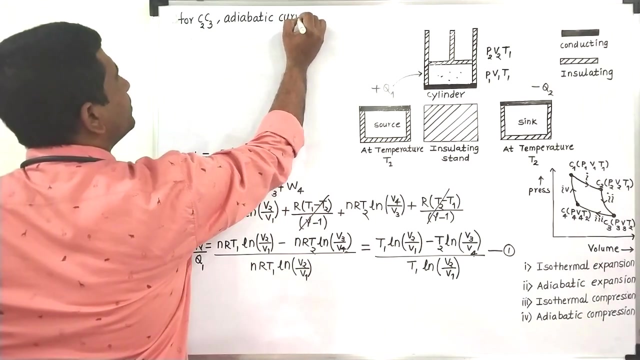 v3, it is at this point v2 and v3, it is in this cycle. c2, c3, for c2, c3, adiabatic curve. c2, c3 is adiabatic curve. it is an adiabatic curve and for adiabatic curve. 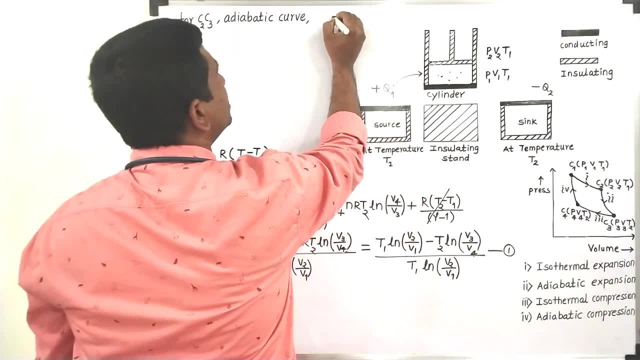 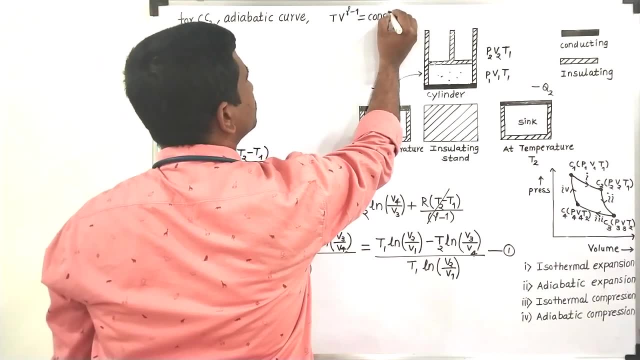 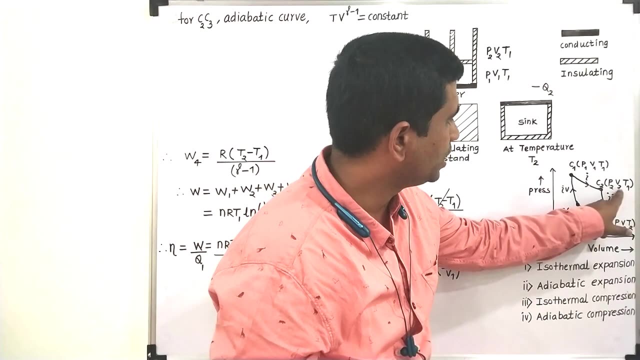 we know the relation. what is the relation? tv raise to gamma, tv raise to gamma minus 1 is always constant. tv raise to gamma is always constant. now see if I say that second cycle, which is adiabatic curve. so in this case volume is: 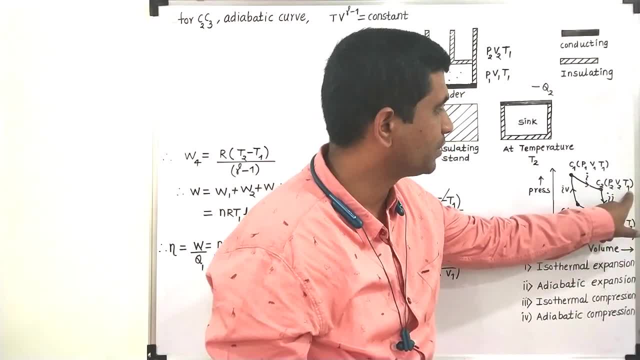 v2, here, in this case, volume is v3, in this case temperature is t1, in this case temperature is t2, so we will write, try to write down that relation for the c3 curve. so it will. 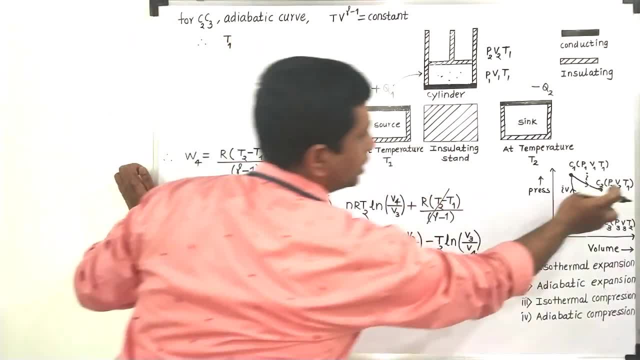 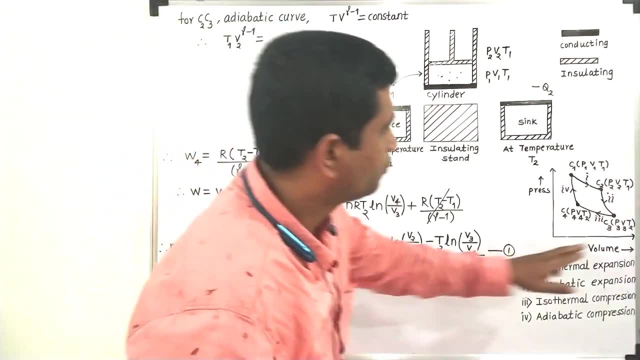 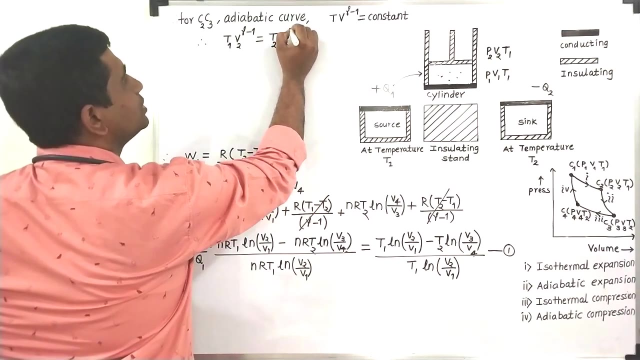 be t1, t1.. v2 raise to v2 raise to gamma minus 1, that is the first relation- is equal to. for this one we will try to write down: t2, v3 raise to gamma minus 1, t2, v3 raise to gamma minus. 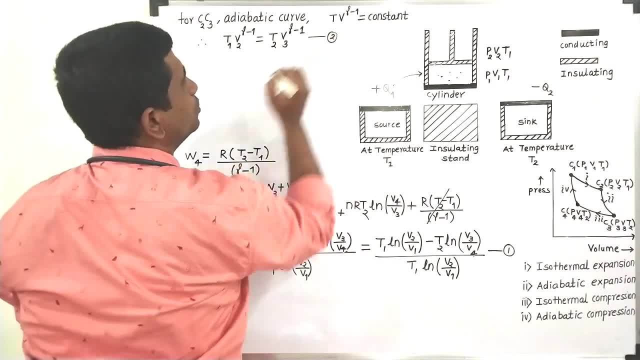 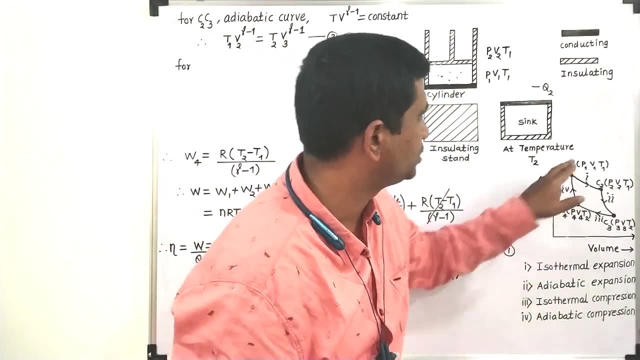 1, that is the relation. let us call this as an equation. number 2, okay for now. next adiabatic curve. it is fourth. that is fourth means c4, c1, for c4, c1, c3, adiabatic curve. 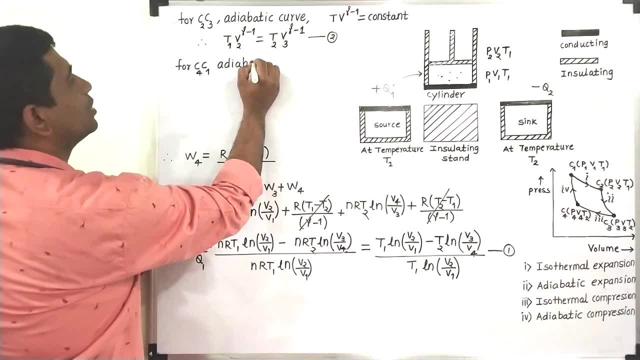 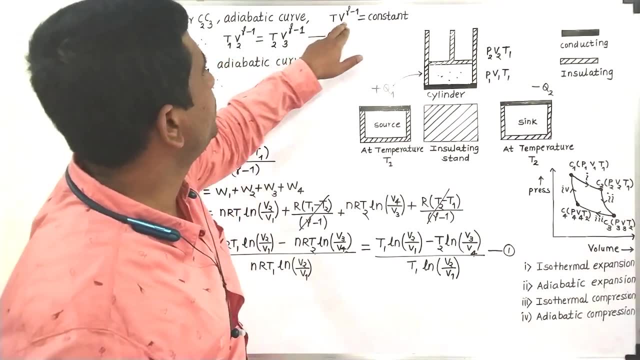 for c4, c1, adiabatic curve. c4, c1, adiabatic curve. why? what do we have? the relation it is tv raise to gamma minus 1, in this case, temperature is t1,, volume is v1, so it will. 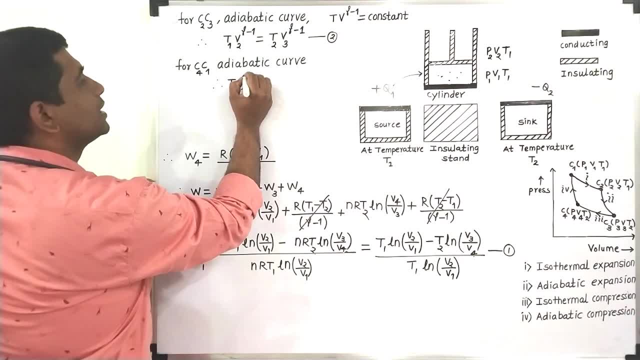 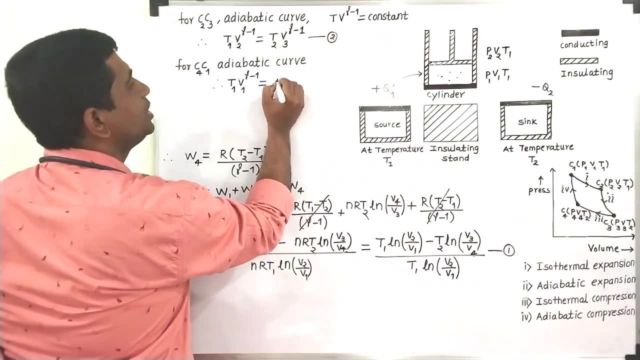 be t1, v1 raise to gamma minus 1, is equal to: and in this case temperature is t2,, volume is v4, so it will be t2, v4 raise to gamma minus 1,, so it will be t2, v4 raise to gamma. 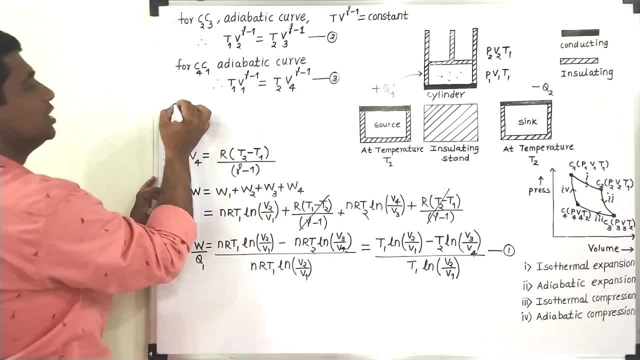 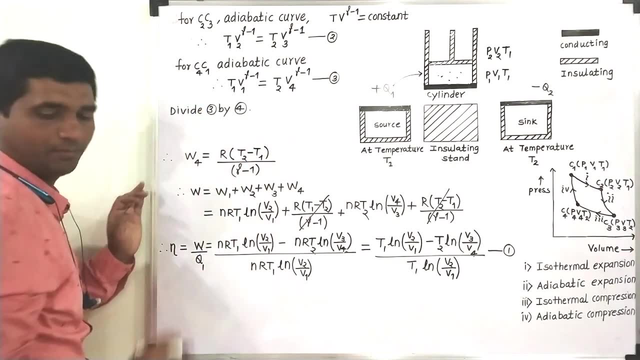 minus 1, let us call this as an equation number 3, divide equation 3 by 4, divide 3 by 4, now if I divide equation 3 by 4, so what I will get if I divide equation 3 by. 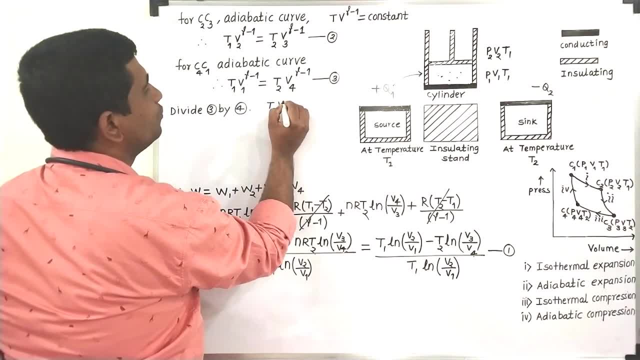 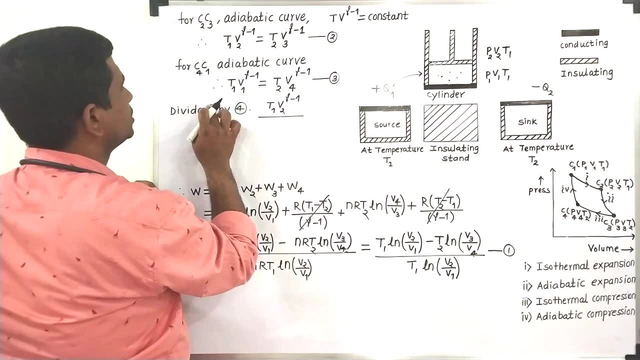 4, what I will get. equation 3 is t1, v2 raise to gamma minus 1,. divided by equation 3 is sorry. equation 2 divided by 3, equation: divide: equation 2 by 3,. 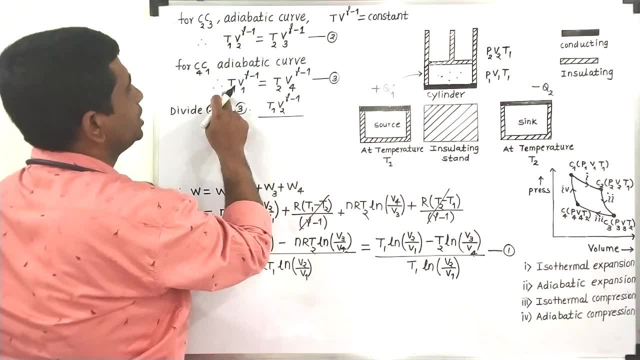 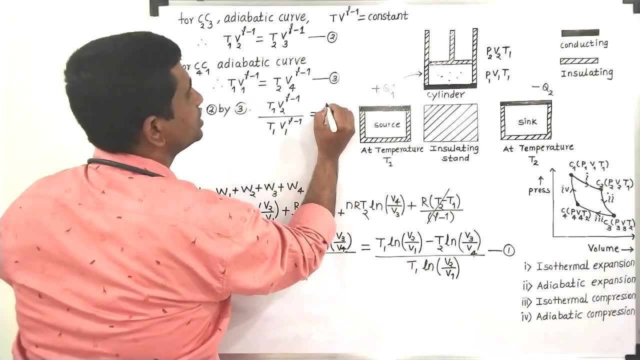 so equation 2 is t1, v2 raise to gamma minus 1, divided by this will be t1, v1 raise to gamma minus 1, this is equal to. in this case it will be t2, v3 raise to gamma minus 1,. 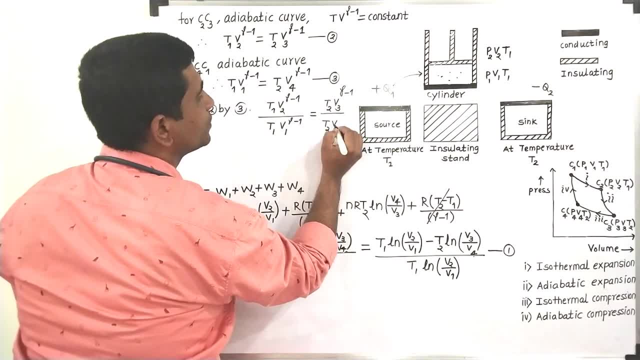 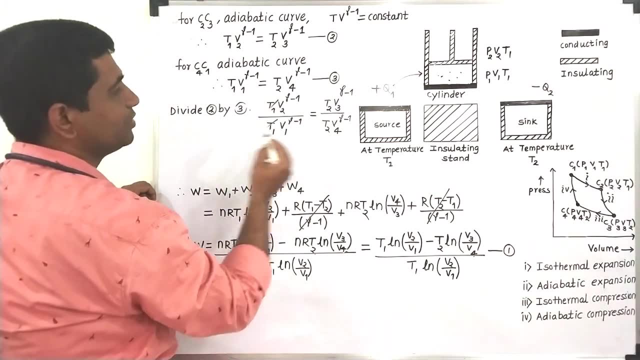 divided by, in this case it will be t2, v4 raise to gamma minus 1,. okay, now see this t1, this t1 will get cancelled. this t2, this t2 will get cancelled, and every time, every. 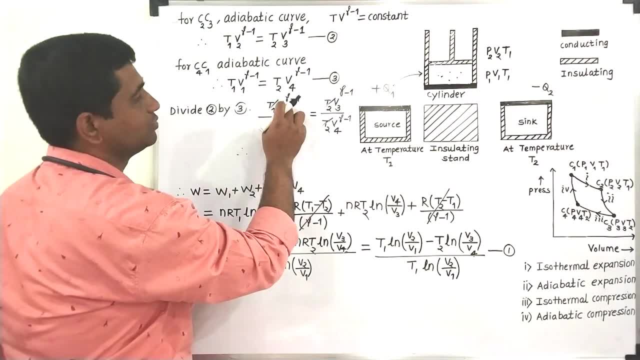 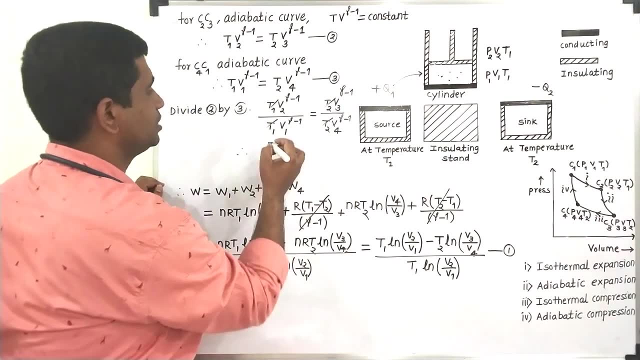 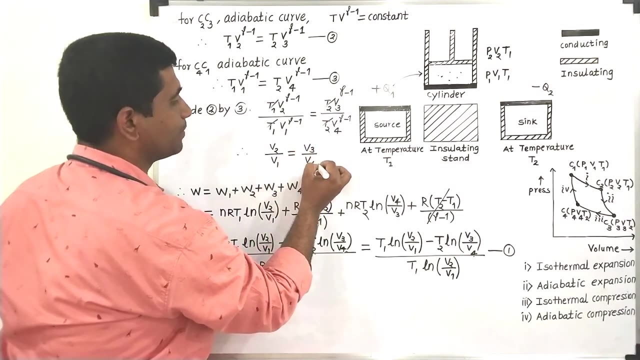 time. everywhere it is power gamma raise to minus 1, sorry, everywhere power is gamma minus 1, gamma minus 1 will take a gamma minus 1 root of this equation. so what I will get from this one, v2 upon v1 is equal to v3 upon v4, I will get v3, v2 upon v1 is equal to. 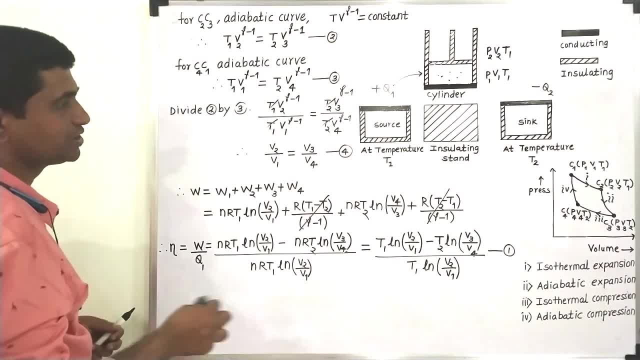 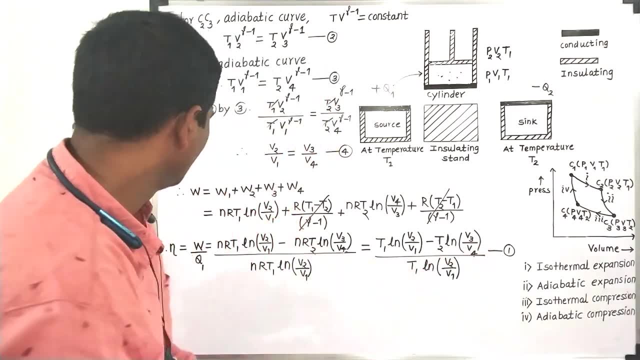 v3 divided by v4, now what we will do. we will substitute this value of v2 by v3 by v4.. v3 by v4 as v2 by v1 in equation number 1, okay, so with this value, if I substitute, 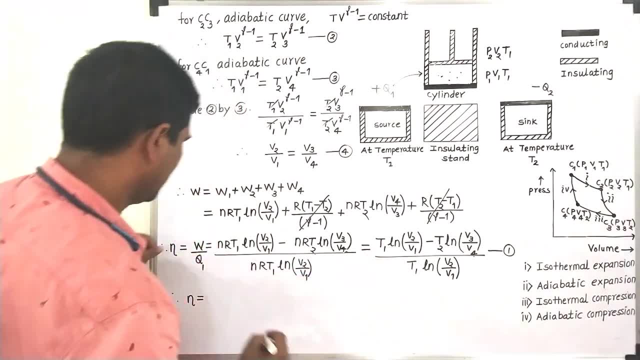 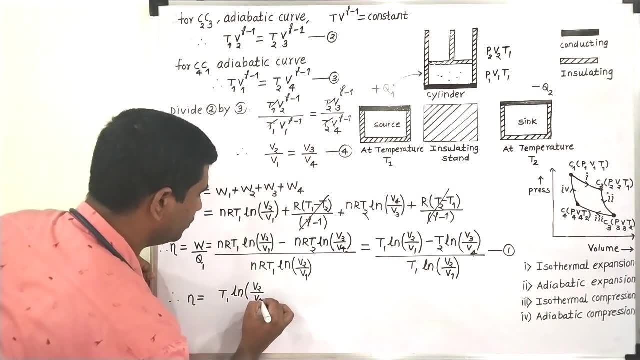 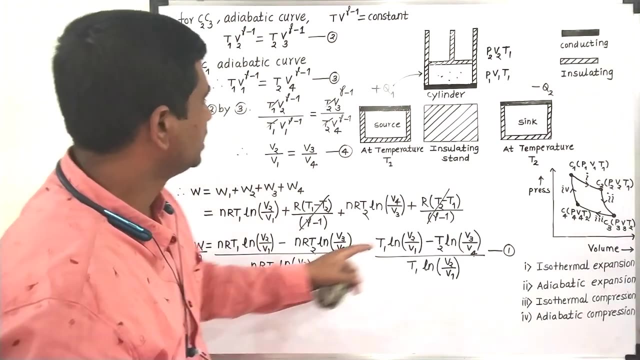 in this equation. so gamma is equal to what will you get? this will be t1 ln of v2 by v1,. this will be v2 by v1 minus. this is t2, this will be t2 ln of, instead of this v3. 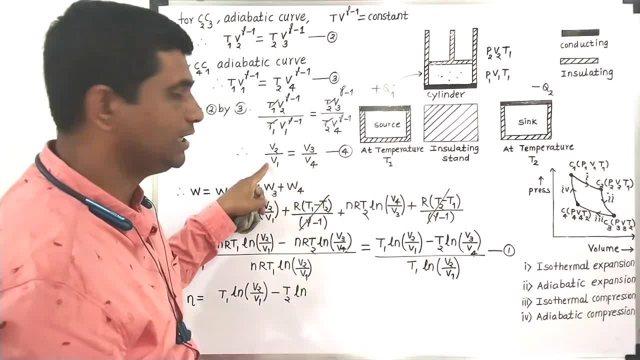 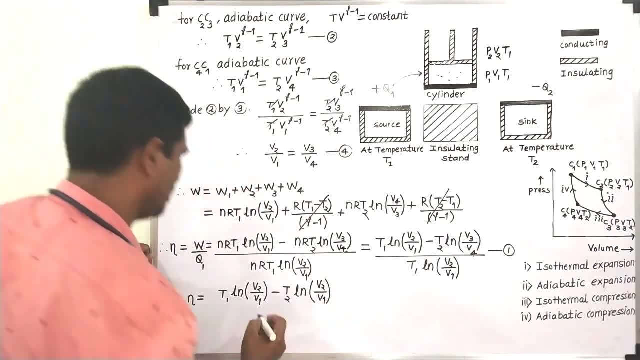 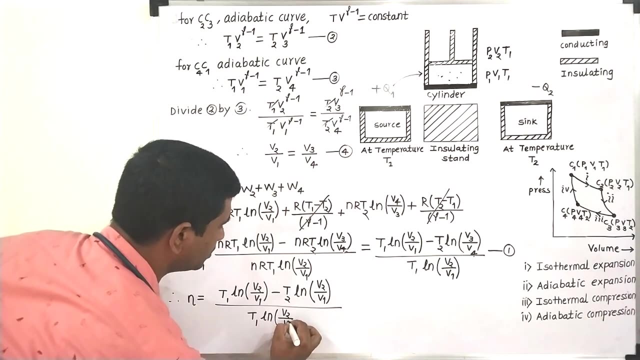 by v4, instead of this v3 by v4, what I will do? I will take v3 by v4, I will take v3 by v1, so it is ln of v2 by v1, it is ln of v2 by v1. divided by this is t1 ln of v2 by v1,. 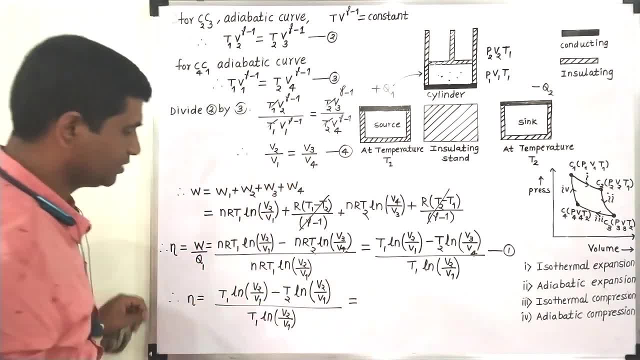 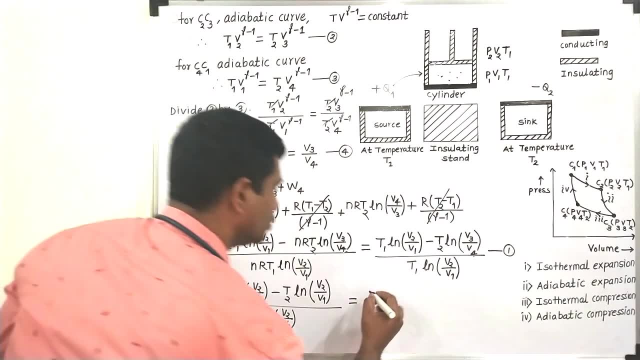 this will be ln of v2 by v1, now in this equation it is ln of v2 by v1, ln of v2 by v1, ln of v2 by v1, we will take it common and we will cancel. so what I will get in? 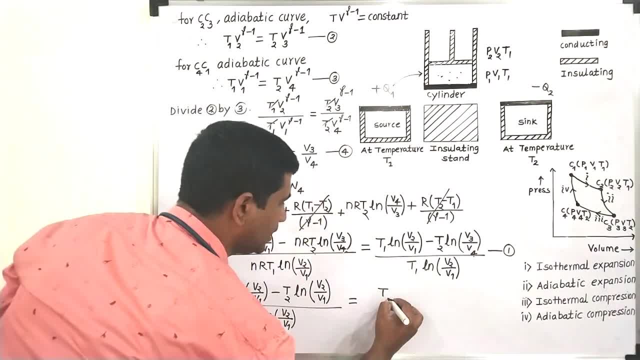 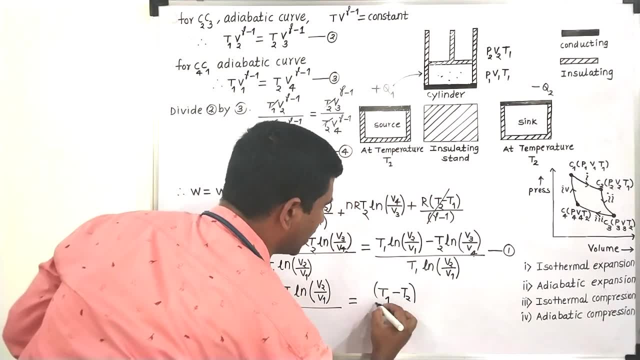 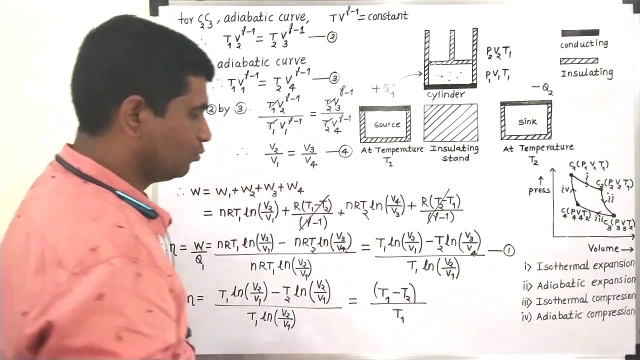 that equation: if I take ln of v2 by v1 common here I will get t1.. So I will get t1 minus this will be t2, okay, and this common which I have taken outside, it will cancel with this one and I will get over here t1, okay. so what we? 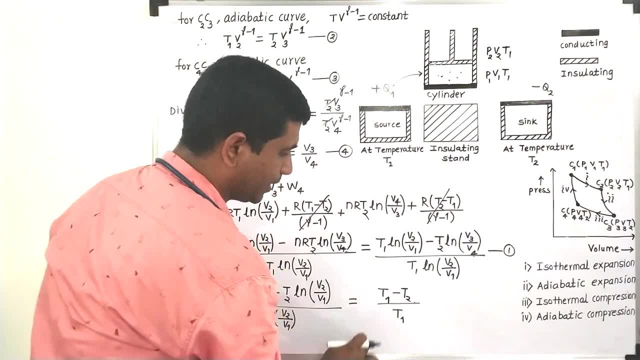 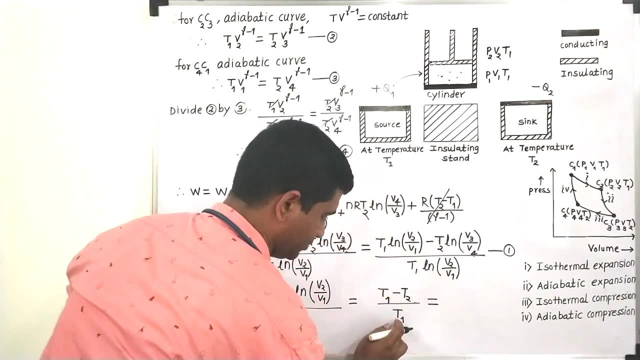 are having is that t1 minus t2 divided by t1 minus t2 divided by t1, so this is our efficiency: if I divide this by t1, so I will get 1 minus t2 by t1, okay. 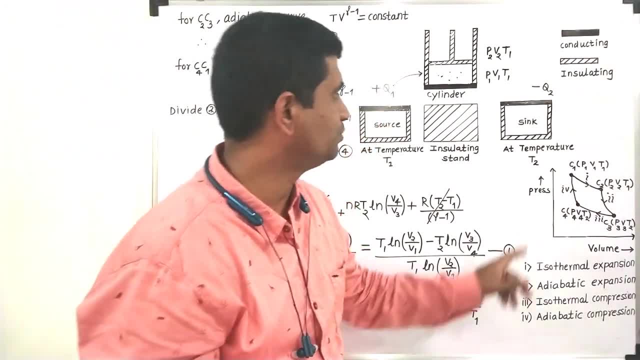 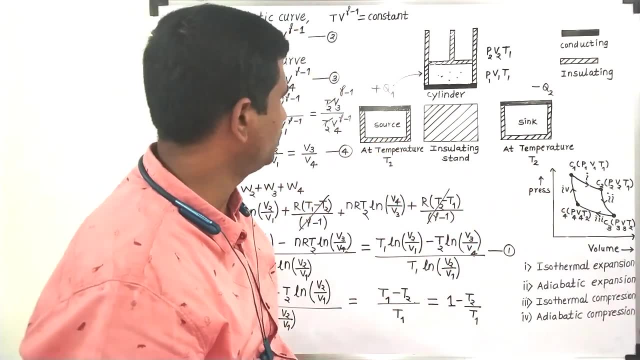 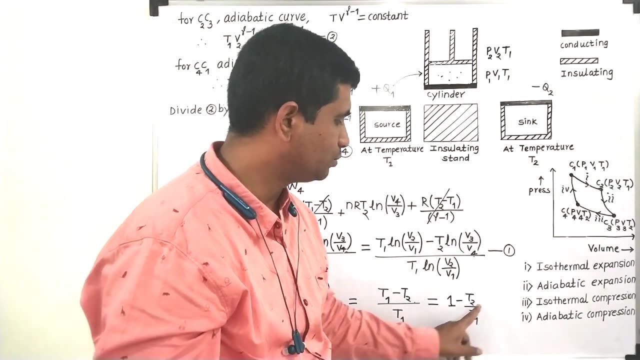 And we know that, as we have assumed that temperature of the sink it is t2, which is always lesser than the temperature of the source. okay, we have assumed t2 is less than t1, so this ratio will be less than 1, and if you convert it to the percentage, this 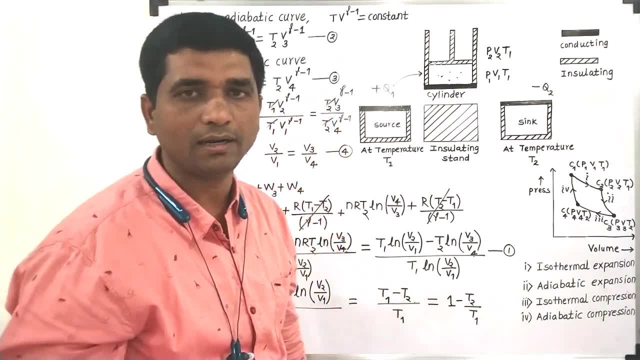 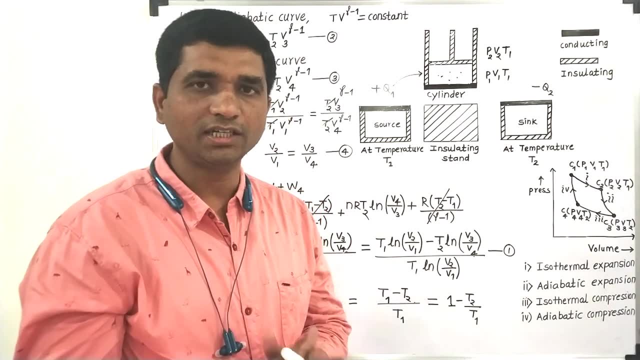 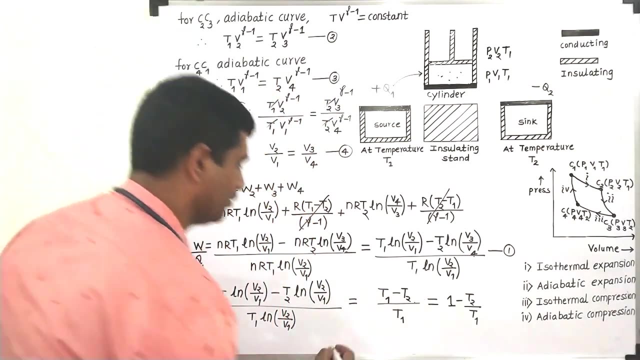 will be the coming out to be 1 minus means it is always less than 100%. So from this expression we can say that it is not possible to have an engine which can be have an 100% efficiency okay in various competitive exams. what you can have is that: 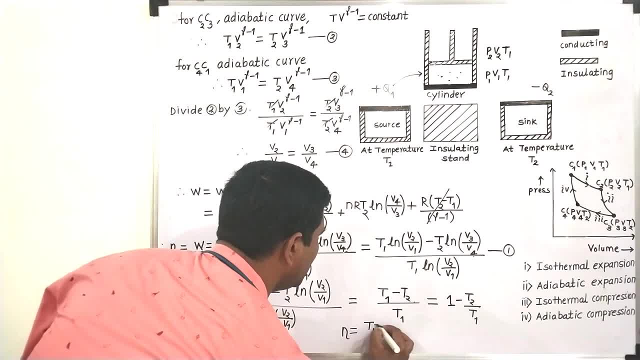 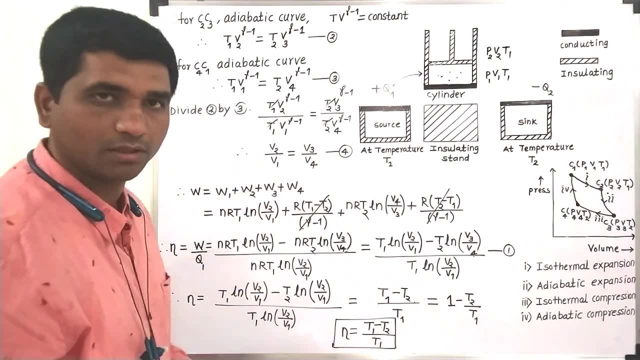 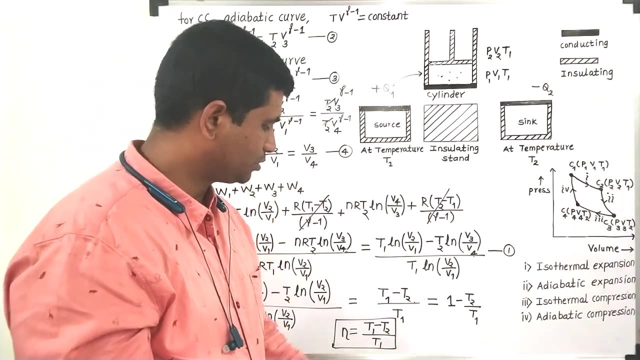 you have to remember this formula. this will be t1 minus t2 divided by the t1, that is the efficiency of a kernel engine. you will get a multiple choice question in various exams or in final exams. also, you can have a question over the numericals based on this.